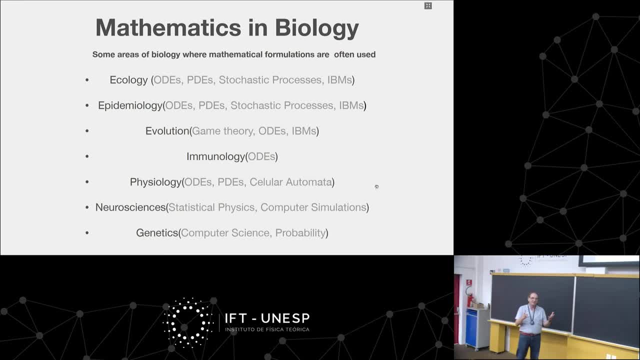 that I understand better. So in ecology you have usually the kind of system you study. you study the population of a certain species, or, and you want to know how the size of this population changes over time and how it changes in space, on the locations. Okay, So this introduces: 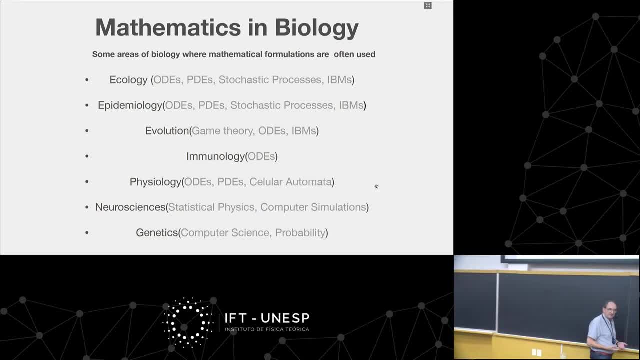 naturally partial differential equation, ordinary differential equations, and to study the populations, Then you want also to study in how interactions between different species modify the population of levels, And and then, well, there are many kinds of interactions. There are the called trophic interactions, which is consumption one species by another. Then there are 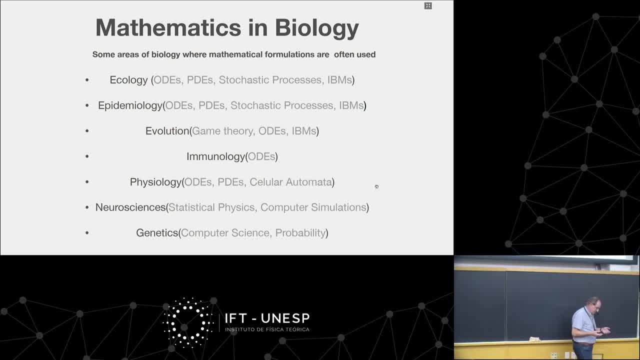 competitive interactions, mutualistic interactions, and all of this can be codified, Usually with ordinary odd partial differential equations for half the number of yeah, svf, and they can also be done using stochastic processes, Stochastic dynamics and also individual based models, which are very frequently used in ecology. 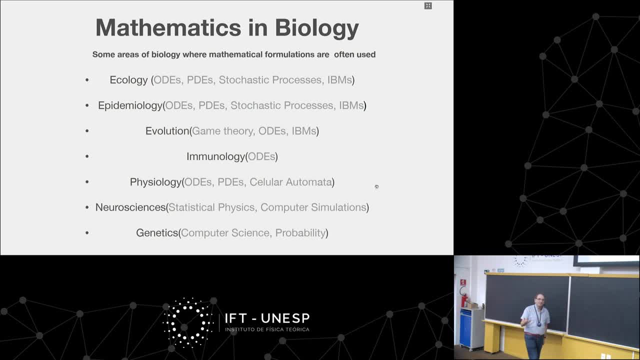 So what are the problems that are of present interest? So there are many, obviously, but one that I want to mention. this is something which is called spatial ecology. It's spatial is collapsing, Is it? No, should it not say: there is no data set that will keep you from. 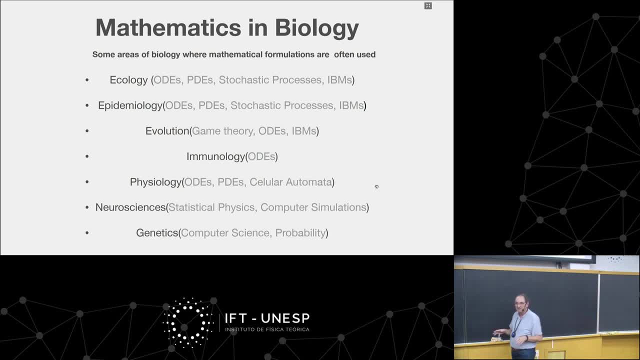 the space spatial dimension affects the populations And in particular when you speak about space and ecology. space is not homogeneous in the sense that space is the habitat, and the habitat may be better in one place than another, Or even there can be places where the population 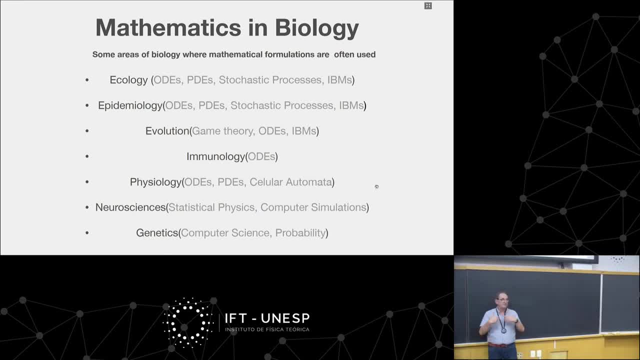 cannot reproduce, for instance, it can only diffuse. So space may be heterogeneous and one very important problem that is being studied is how the fragmentation of an habitat affects the population levels of the species, affects the equilibrium between different species. How can fragmentation promote invasions by alien species which may be they are better? 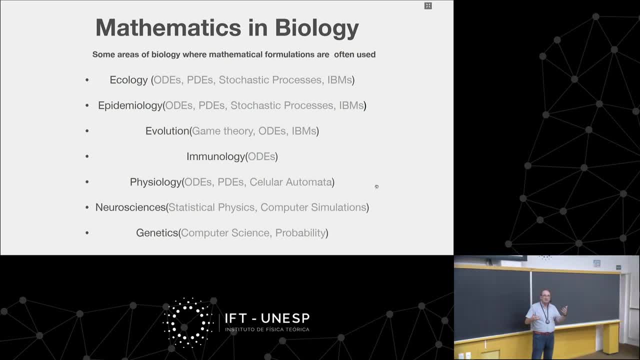 for instance, in fragmented areas, because they can maybe cross from one fragment to the other They are easier than the resident species or something like that. So this is one of the focus subjects that are being studied in spatial ecology and it's very applied. 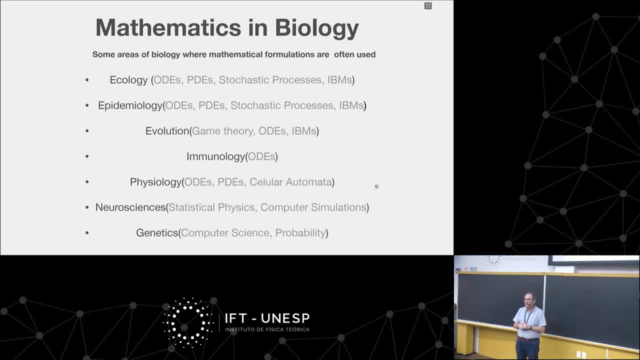 also because fragmentation is very widespread. If you look for the Atlantic forest here in Brazil, it's essentially a fragmented habitat and all small, small fragments, and then they have the species that live in these fragments and they cross the fragments and then they are ones that can cross easier than others. 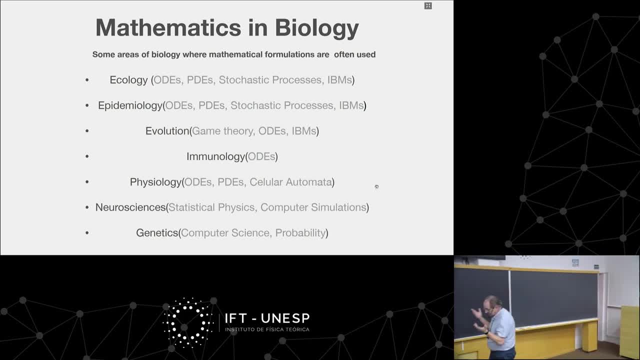 So in epidemiology there's also this kind of mathematical formalism that I have just written there. I will discuss this later, because that's what will be the focus point of my seminar in a few minutes. Then there's also the discussion of the relationship between the species and the environment. 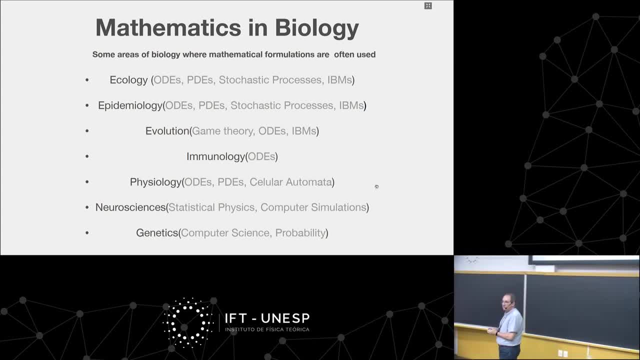 There's discussions, mathematical modeling of evolution, which goes usually through game theory, and also ordinary differential equations and individual-based models. Individual-based models: so you have this computer model where you consider individuals and they have rules- how to interact or to move or take actions- and then you put a lot of individuals and 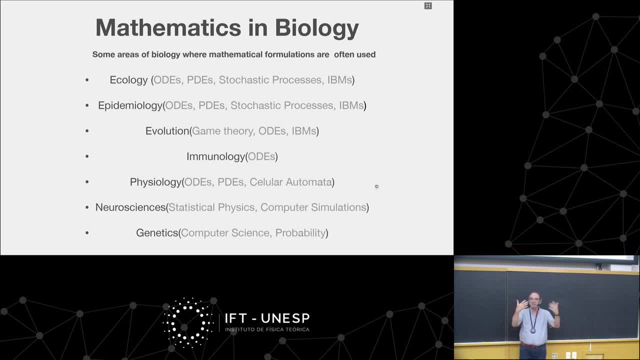 then you run, You run programs, run the code to see what happens with this population under different constraints. So to give an example of what is important in evolution that has been studied mathematically, for instance, is the process of speciation. Speciation means the production of new species. 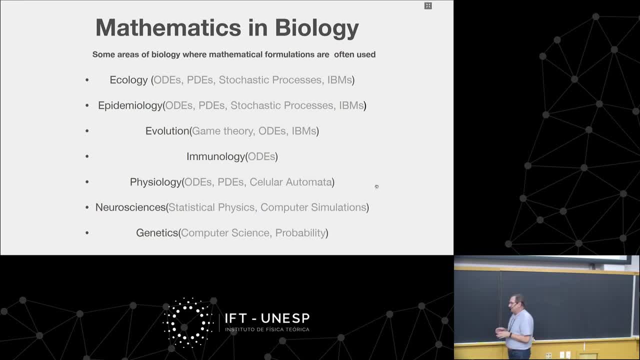 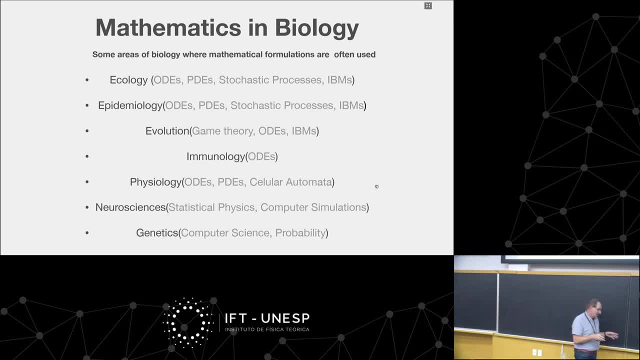 But how is this process going on? One of the things is that there are many ways to have new species. For instance, one is geographic separation, So the species on one side of the mountain and the other species on the other side of the mountain- they cannot cross. 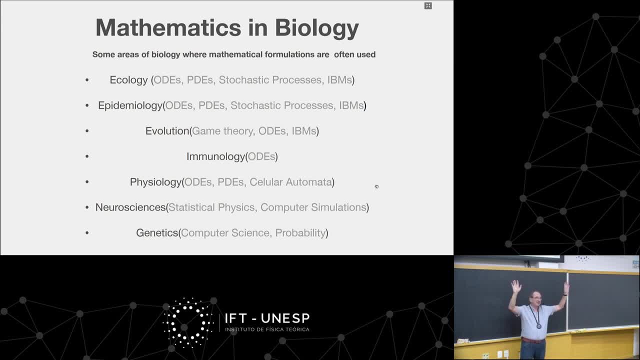 They will go on, will go on the evolution for a long time and then they at a certain point they are not made anymore the same species. that's the classical. it's called a pyropathic speciation. but then there are. there's process also which involves 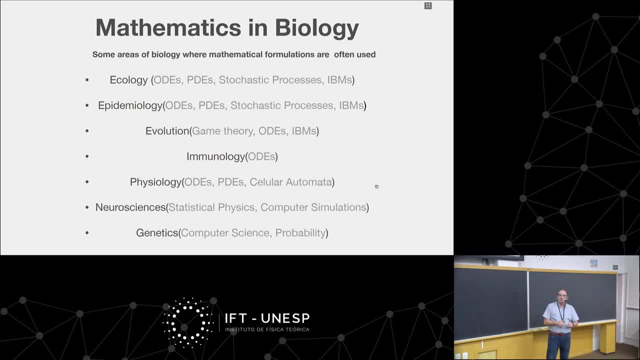 natural selection. but there's also something which is called genetic drift, which is just having a species in a certain region that can move and can reproduce, has a genome and has some mutations, which are rare, but over time they may accumulate, and then you have, without any spatial separation, you have 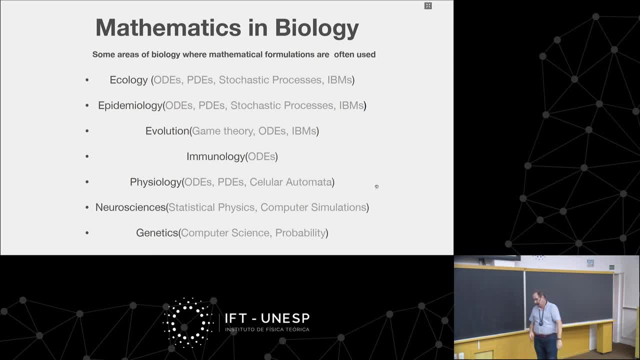 new species appearing. so this is a work from specialist of. this is one of our, our friends, Marcus Aguiar from UNICAM. Immunology is something where it's studied like population biology, but with different laws, and it's a very interesting study. because it's a very interesting study. 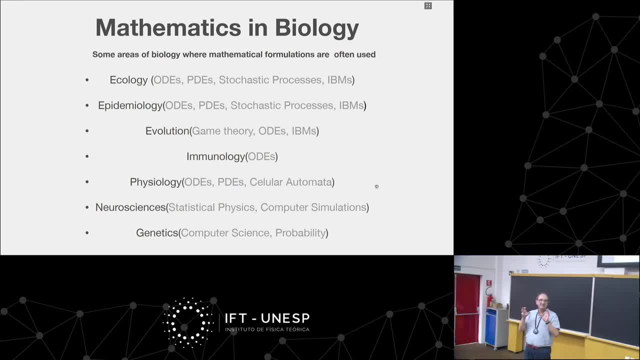 because when all the elements of the immune systems are given in terms of concentrations and then in reactions and so on. so I won't talk much about this thing because I don't work with it. physiology is also a subject where mathematics is important, for instance for modeling of cancer, cancer processes. 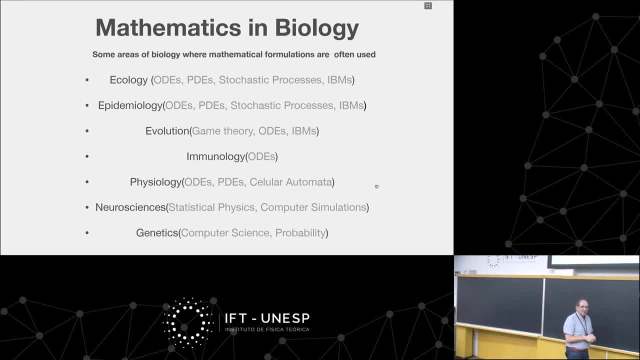 in your body. okay, these are usually kind of reaction diffusion equations. you have the diffusion and them and of certain species at certain kind of cells and so on. so that that's one, but that could also be a physiology, can also be some more microscopic things like like abilities to like biomechanics and so on. 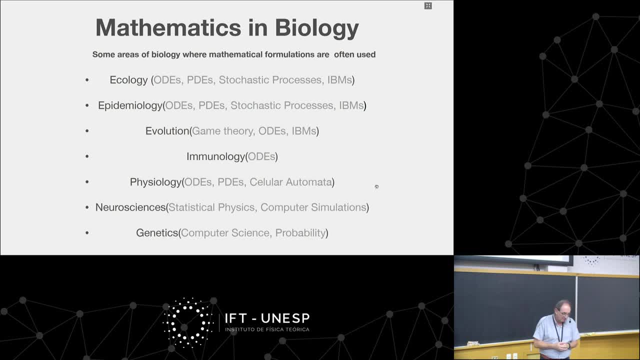 right abilities to fly or to walk and so on. So that's a very interesting study, which is a study that can be done in a complex way. Neuroscience over the last 30 or 40 years has come to rise as one very important area in biology. 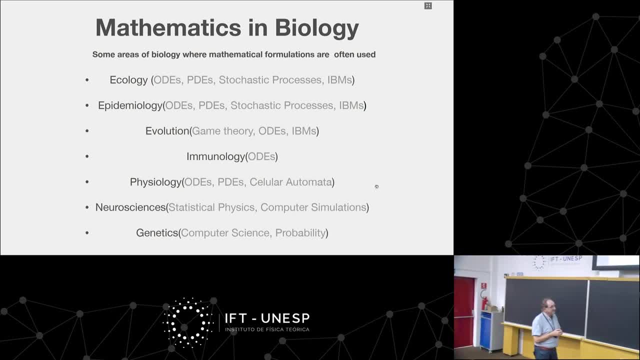 There's a lot of work going on with statistical physics and a lot of computational work, and I would say it's still at the beginning of this subject. And then obviously, genetics, which is a little bit different from the usual setting of differential equations. 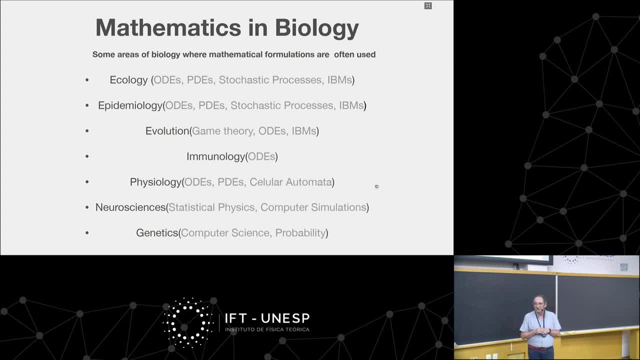 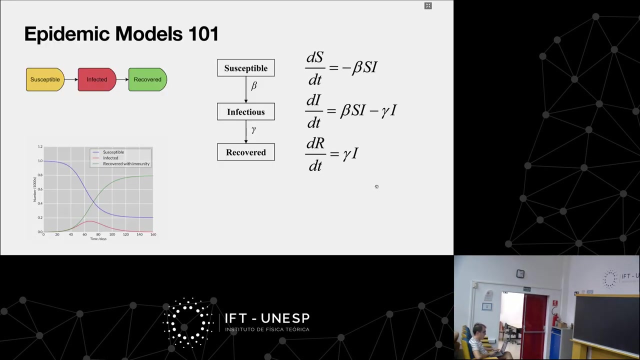 It's much more about computer sciences and probability and this kind of thing. That's a very general view of areas where mathematics has been successfully used and has given contribution in biology, In the biological system. it's not exhaustive, obviously. Let me now talk a little bit about models for epidemics. 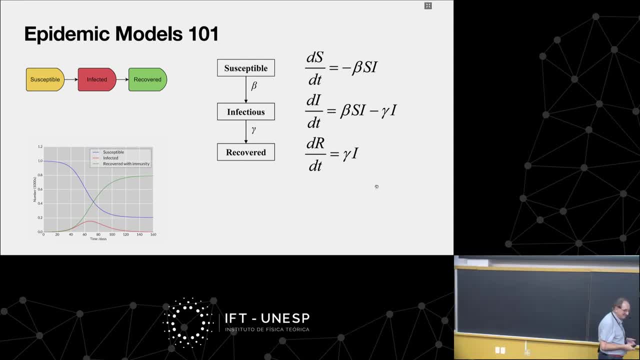 Epidemic Models 101 is something that most of you have probably seen, Due to COVID and so on. everybody has heard about it. But just to mention, usually what you have is you take a population and you divide the population in classes. So with respect to their state, with respect to the disease, 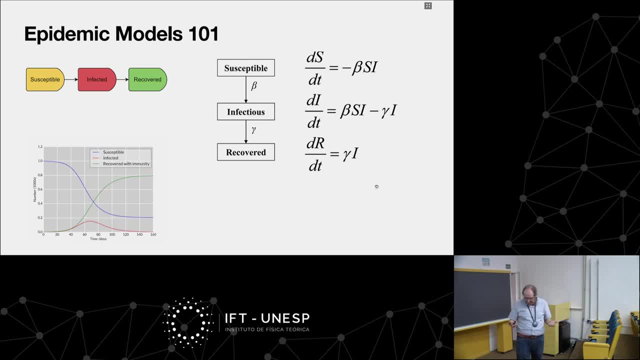 So you can be susceptible, which means that you can catch the disease, You can be infected and infectious at the same time. You have the disease and you can transmit, And you can then get recovered, And this is usually modeled by ordinary differential equations. 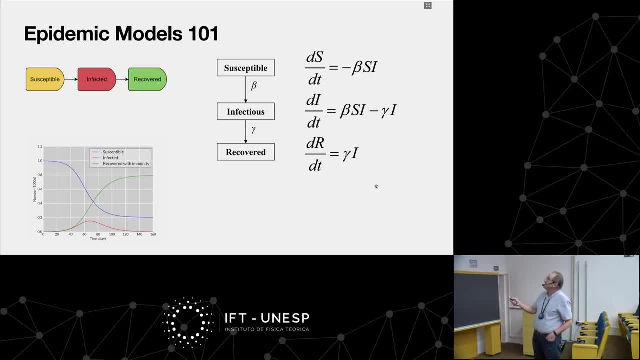 You say that the rate of change of susceptibles over time is something proportional to the number of susceptibles times the number of infectious people And all of these that are susceptible and leave the susceptible class go into the infected class And then after some time they will leave the infected class to go to the recovered class. 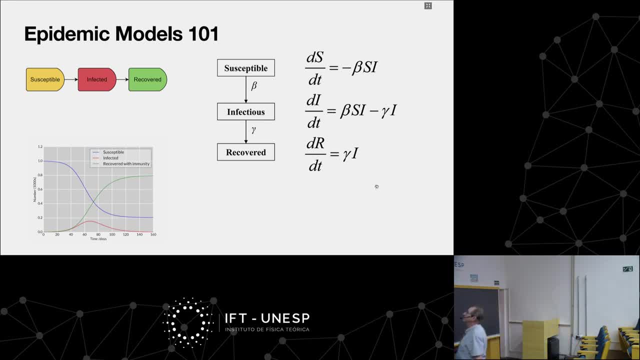 They can die also. yes, Well, in this case I'm taking the case well, this is a closed population, for instance. So if you want to have a system where people actually die, they are born also. So usually most models will look at this as a balance between death and birth. 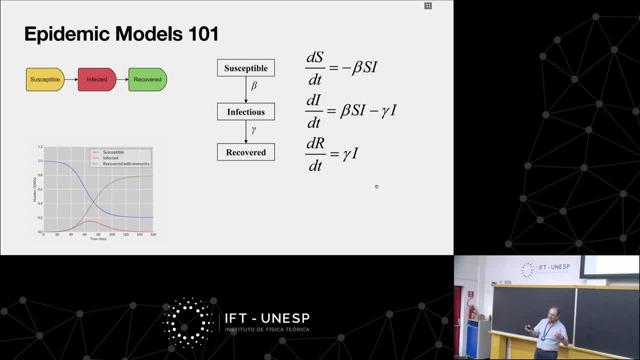 So the population stays constant, Which simplifies the problem, And this is usually okay, because the change of the population to be important takes many years And usually epidemics don't take many years, So it's a good approximation. 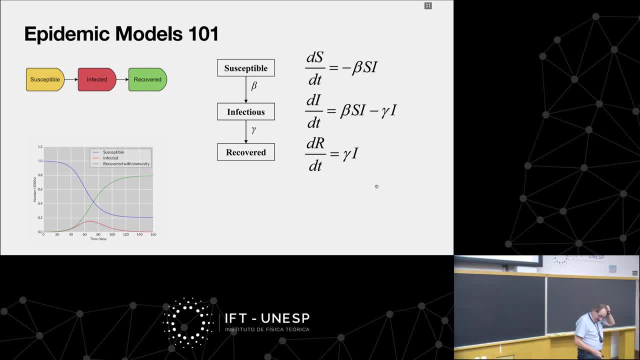 So well then you get it probably. Okay, this is the solution to this equation. So you start with everybody susceptible and epsilon, a very small number of infectious people. Then you have an infection and a curve of up and down, which is the number of infected people. 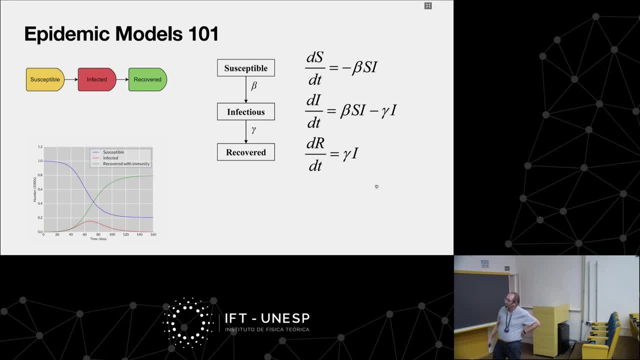 Susceptibles decrease and the recovered only increase. And you see that at the end in this example, at the end, when the number of infected people already got to zero, you mean the epidemic is over. they're still susceptible people. Not everybody gets the disease. 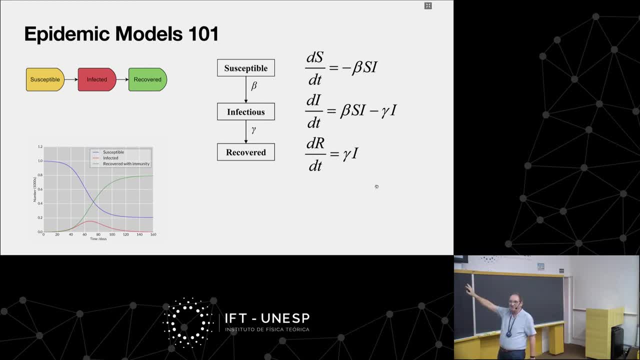 So this is the for this simple model. the main result of this simple model is that not everybody gets a disease of this kind. if it's an SIR, Obviously. if you don't have recovered people and people just get back to being susceptible. 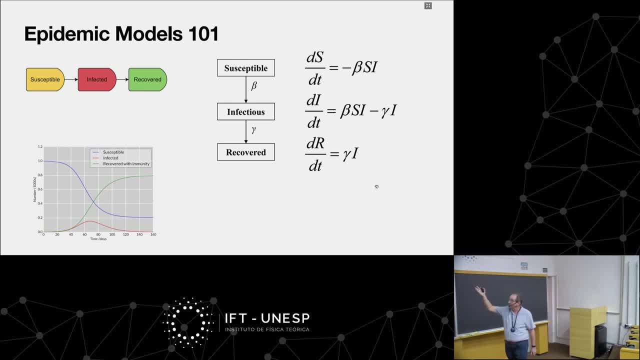 then you can have everybody with the disease. But if you have recovered people, then not everybody gets the disease, And so this is kind of burnout of the epidemic. So more complicated models. you see more, more compartments. Maybe you have people that have been exposed. 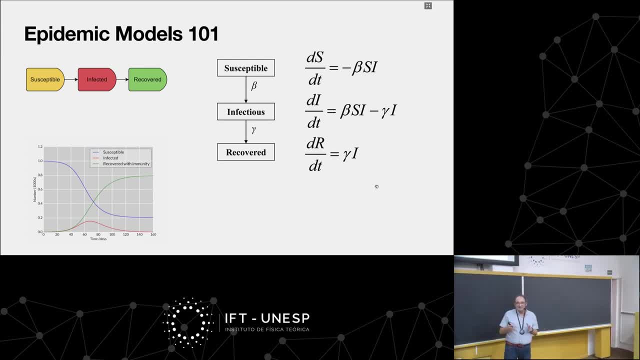 They are infectious but they don't have the symptoms. You separate this infectious into exposed- And if you want to call it asymptomatic, it depends a little bit- And then you have the infectious people that are actually infectious and infected and have the disease. 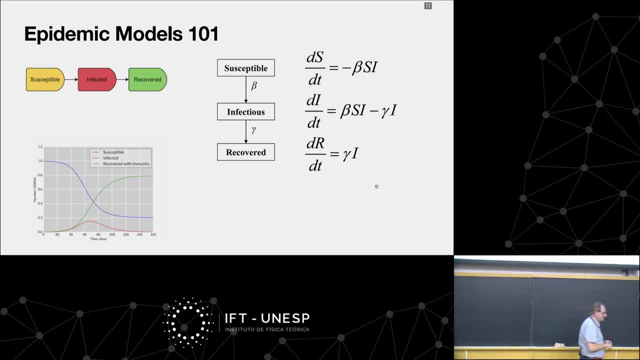 So this is something which is easy to do. Then you can have partial recovery, recovery after sometimes people lose immunity. Then you get recovered, going back to susceptible. Well, And for models that are actually something which is useful, you need more classes. 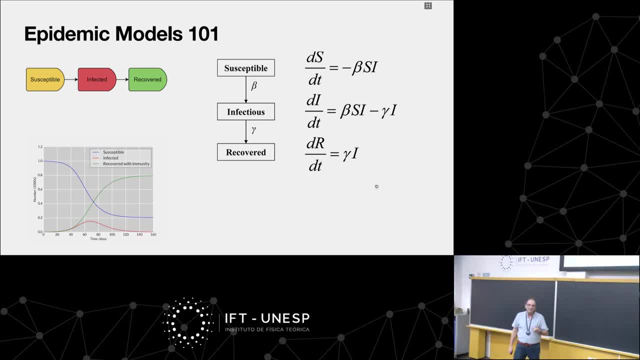 For instance, hospitalized people, Hospitalized people, asymptomatic, and so on, And depending on the pathogen you are studying on the disease, maybe you need to take each of these compartments and divide it by age classes, For instance for COVID. this is important. 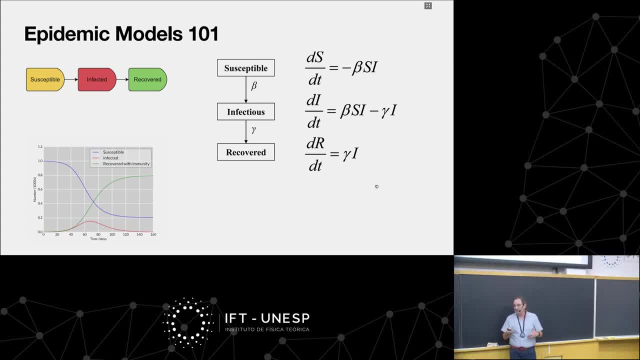 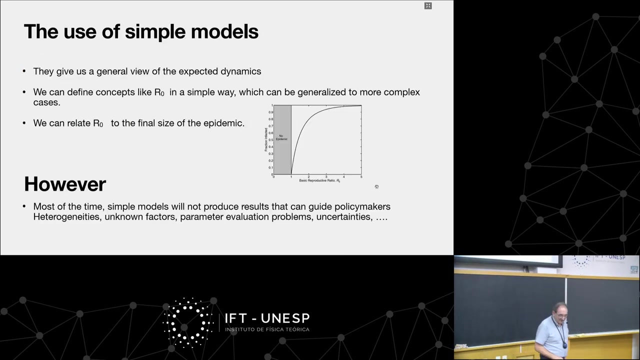 because the effects of COVID are different in children, in adults, in elderly, and the rate of death is different. So you have to divide your population by age classes. So this makes the number of equations grow very fast. Okay, So there's a problem. 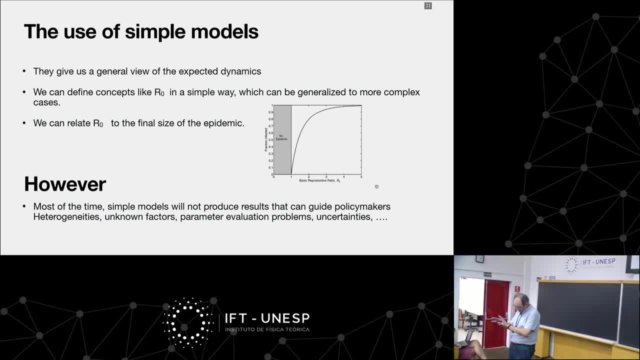 You usually want to fit the lowest number of parameters you can. So you have things that you have from data, from observations. There are things you know under the range. So all of this, I won't go into this, but all of this has to go through an analysis with error bars. 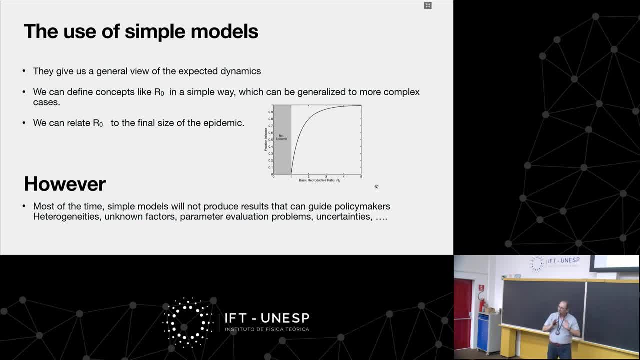 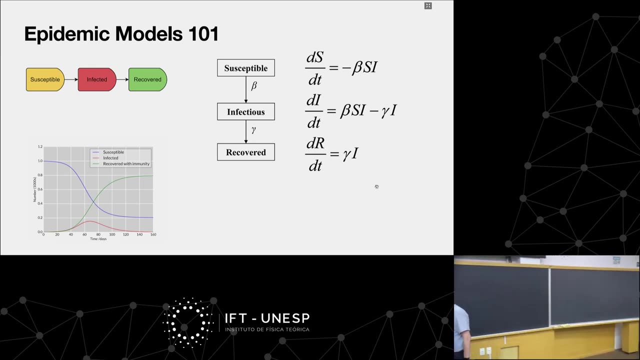 with everything. so, in order to make sense, Okay, And one parameter that you never know is the beta Okay, Which is you can think it's proportional to the probability that, if a susceptible person meets an infected person, what's the probability that the person 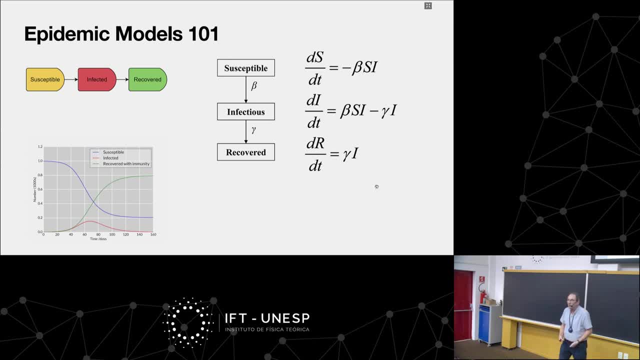 the person gets infected, right. So this is not. you cannot know this beforehand. So beta is always fitted in the models, Okay. What you should do, however, is not to do overfitting. Overfitting is very, very bad. 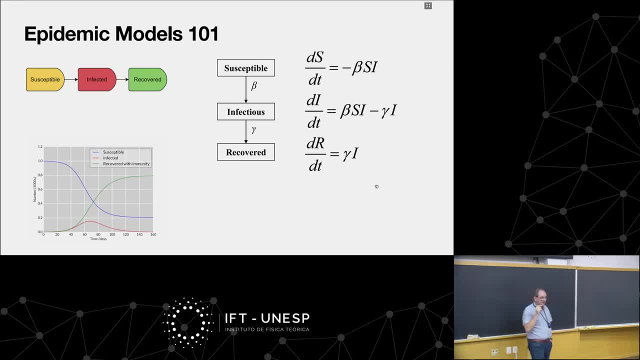 So one typical overfitting problem is people that go here and say that okay, let beta depend on time, And then every step I fit a beta in time. If you are doing this on a daily basis and over one year, you have 365 parameters. 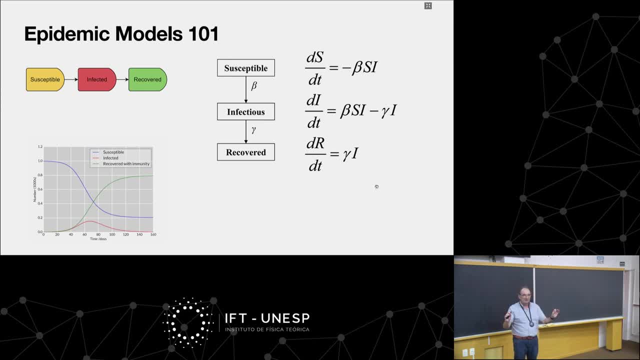 which is overfitting, which will fit perfectly the curve but will predict nothing at all, Okay. So there is a kind of art of being reasonable with the fittings, Okay. So usually you'd say I want a beta that is either constant. 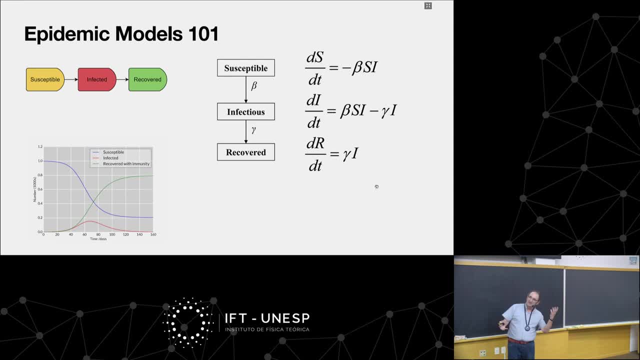 or maybe in the winter it's a little bit higher than in the summer, but not fitting it every day or every week. Okay, Yeah, No, So predictions. so that's something that people. influenza is a very difficult disease to study. 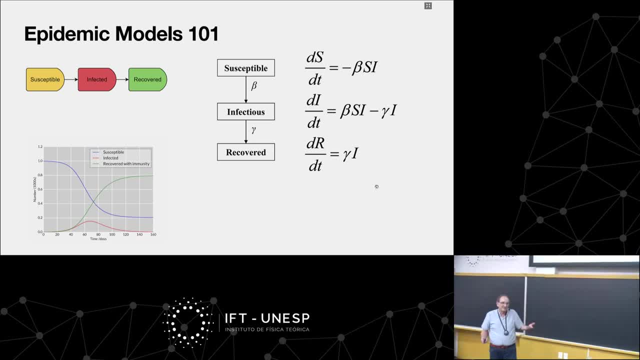 because you don't have good data, Because if you get the disease, you stay at home and it doesn't go to any doctor, And therefore, why you don't? the public health data does not show it. Okay, What public health data will show is: 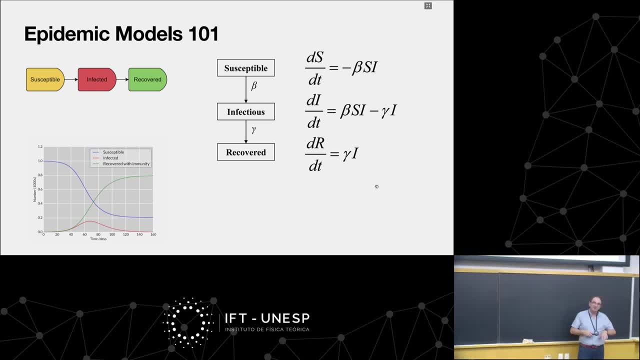 is hospitalization of people. Okay, So that's a proxy. And so there are people that have run very big programs that take everything they can into it's Google search, it's climate, it's everything you want, and machine learning things. 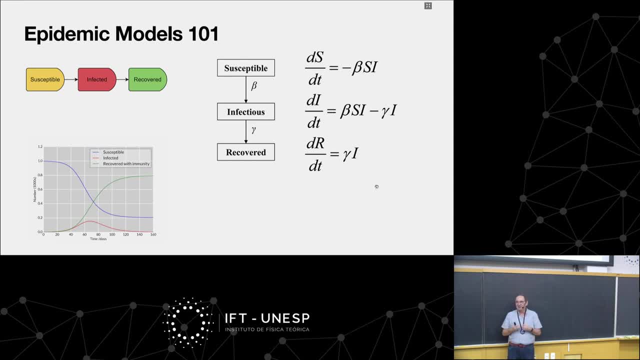 and trying to predict the next season, But not the number of cases, it just will be important or not, and so on. The same thing is, for instance, dengue, Dengue, what we have here, and then that's actually something that we are working at. 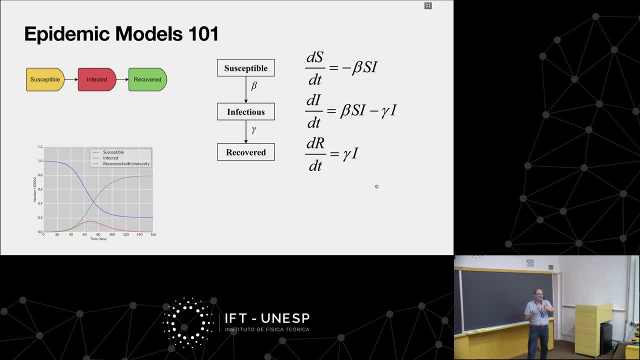 is to try to say what makes that some years you have much more than other years. Is it just climate? But it's not just climate. Okay, There's something else. So what are the, the motors of this? It's usually difficult to understand. 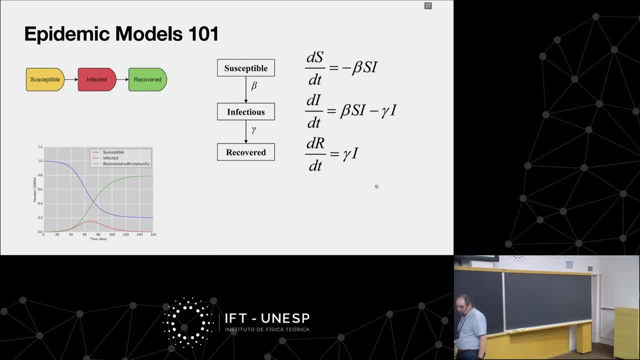 Okay, And it would be very important to understand, for instance, if you talk about influenza or even dengue or anything, because even if you cannot avoid it, sometimes you can prepare the public health, hospitals and so on. This year we need more. 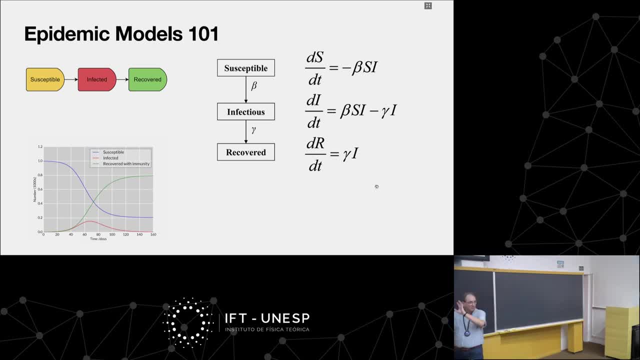 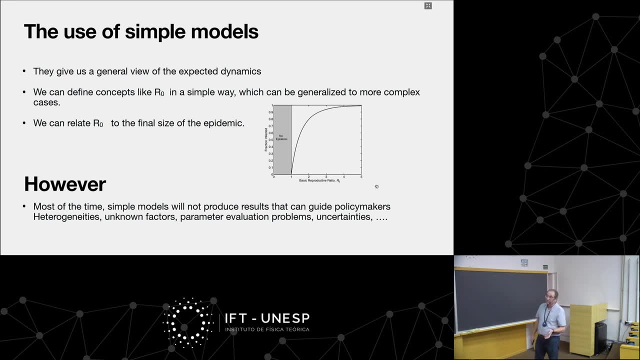 more beds or whatever, more doctors. So that was a very simple model what I showed. and this model is good because we can define one important parameter which is called R0, which is the reproductive number, The basic reproductive number. 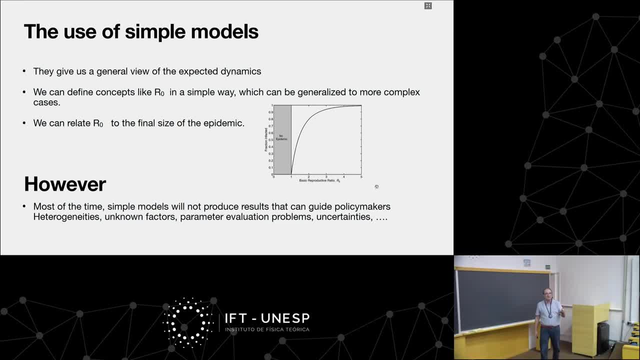 which is the number of secondary cases that one primary case creates Okay. So if R0 is bigger than one means that you have an epidemic, because each case creates more than one okay in average. And one thing about this R0 is that in the simple models, 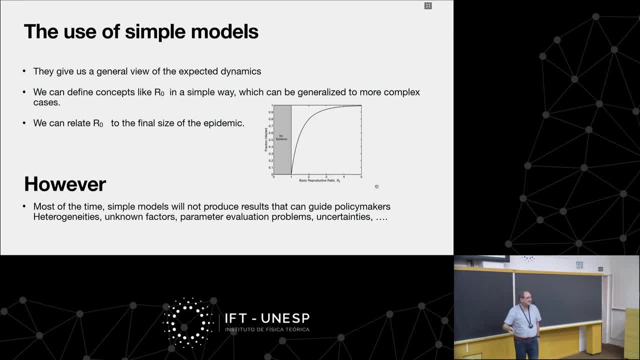 you can relate R0 with the final size of the epidemic. What's the final size of the epidemic? The number if the epidemic goes extinct. after it goes away, there would be a certain number of people that had the disease And this is called the final size. 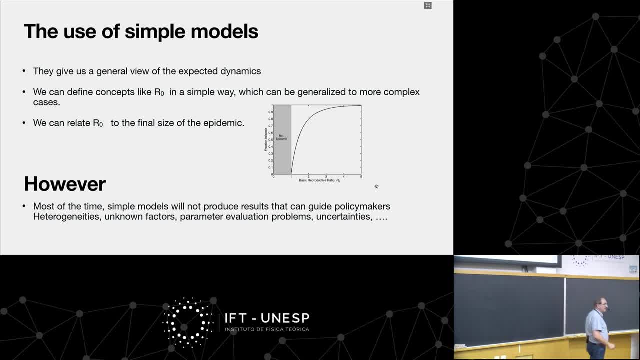 Okay, And the final size is connected to R0.. It's a very elegant result for many, many models And it's something a curve like that. Okay, So that allows you to say if I have measured. but at the beginning 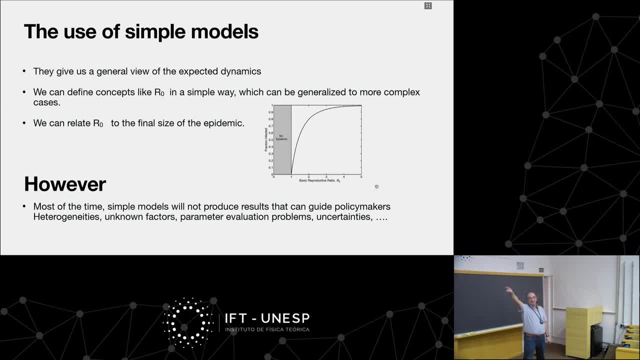 R0 can be measured at the beginning, Right, It tells you something about how bad things can be in the future, Right? What's R0?? R0 is the number of secondary cases that one primary case will infect. Okay, So, 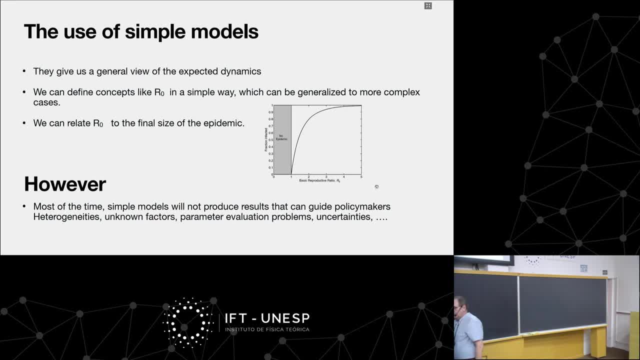 on average. No with immunity, No with immunity, But wow, okay At the time. zero, no immunity. So F is, by definition, constant. R0 is, by definition constant. R0 is is. no, it's not constant. 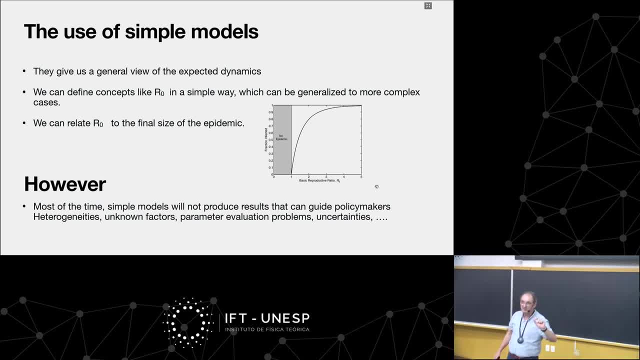 R0, I mean people. when I say at the beginning there's no immunity, immunity will build up because people will get immunity. Okay, So the number of secondary cases that a primary case will infect will depend on time, which is called the RT. 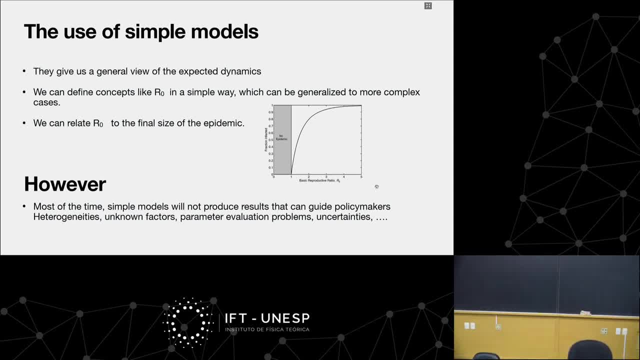 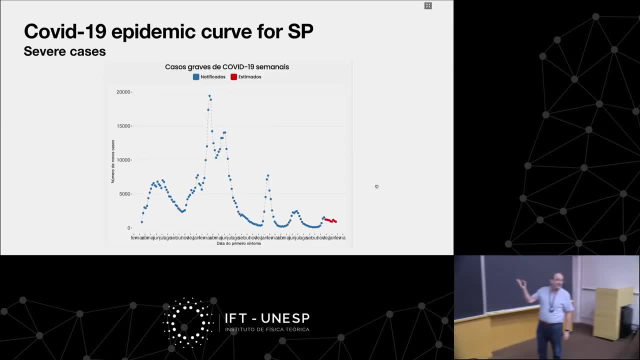 Okay. So one is: the R0 is by definition constant. Okay, So this is the R0.. Okay, Um a, so R1, the R1 is by definition constant. Uh, uh, Okay, But. 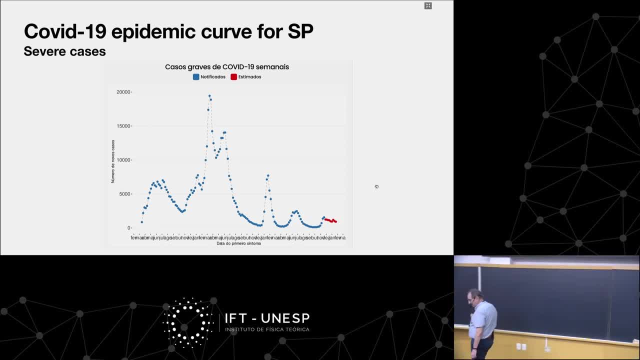 uh, we are, uh, we are always like that, Nothing like the beautiful curves. Yeah, This is the uh, uh, covid-19 epidemic curve in Sao Paolo, And it goes up and down and you see that. so, and here this is again, it's on the severe cases, because for COVID-19, 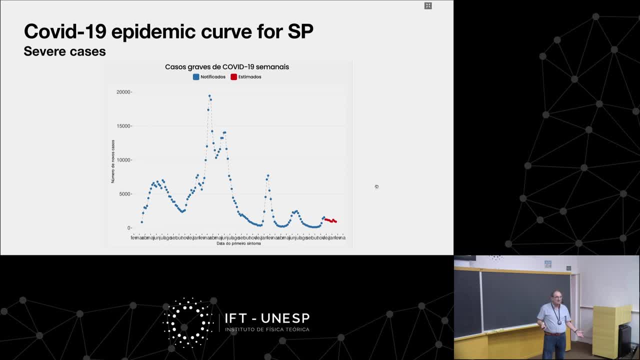 we don't know the number of cases if people look at the disease and it's not notified by the system, even if they go to a hospital or to a doctor. if it's a mild case, then it's not notified, so it doesn't get into the system everything. 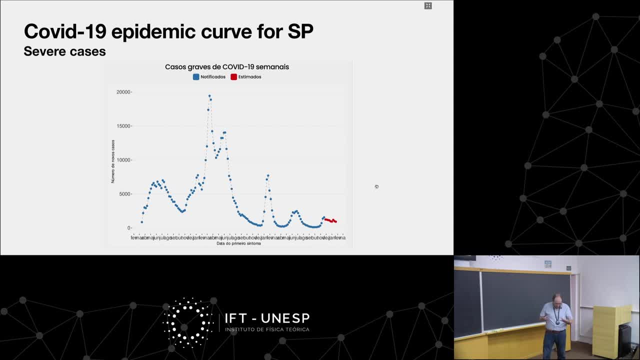 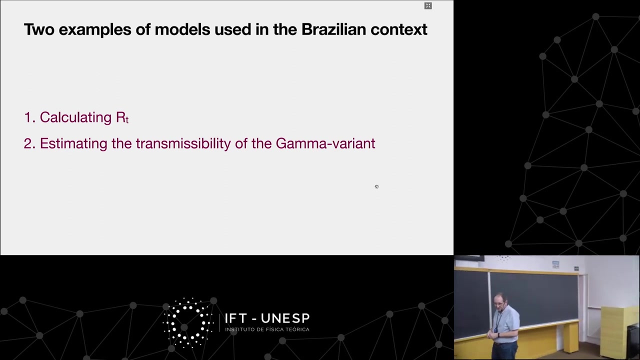 that goes in, I mean, most things that go into the system of notification are hospitalized case, and that's what we have and as a data that are they can we can actually work with. so now come on. okay, let me give you very shortly two examples of models used by our group worked on. 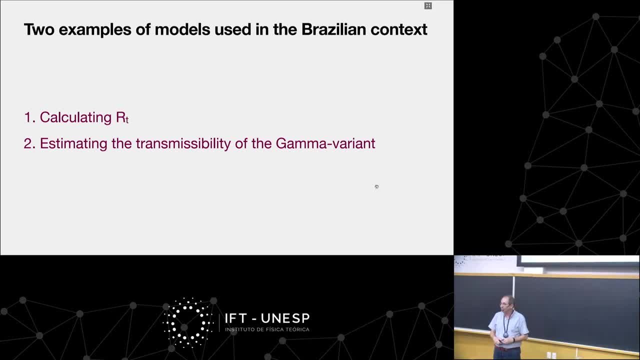 and give you some take what the kind of problems that we have worked in in the Brazilian context. I mean Brazilian context, data from Brazil. so first is calculating RT. RT is the number of secondary cases that the primary cases infects at a certain time of T. so our zero was at the beginning and this is 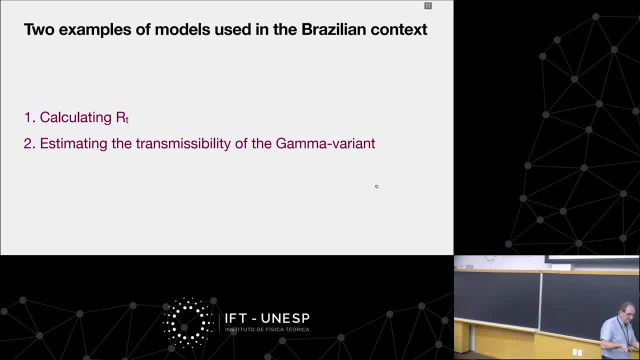 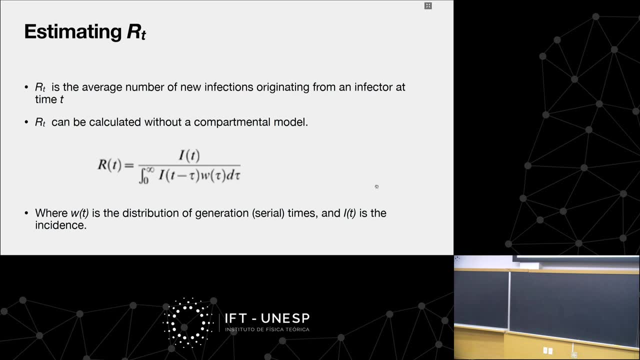 the secondary, it's at a certain point of time. okay, so, and people were eager to estimate this, always because they want to know it's bigger or not than one. okay, are we already decreasing? I mean, what is the situation? and so the first thing is RT. it can be calculated without any. 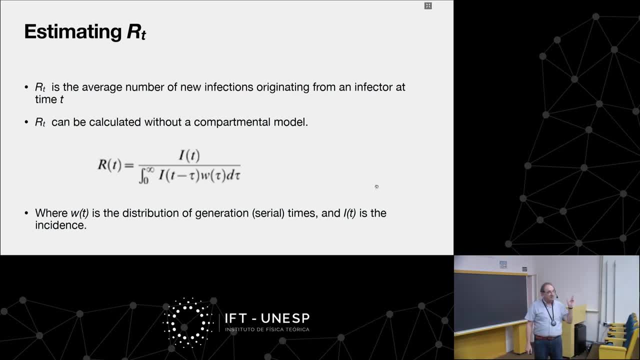 model. actually, you don't need a compartmental model. you just define RT as the number of secondary cases that the primary cases infects, and then, with some elegant mathematics, you come through this expression where I, well, I should not have used: I here. I is not the same, I as an SIR, I is the 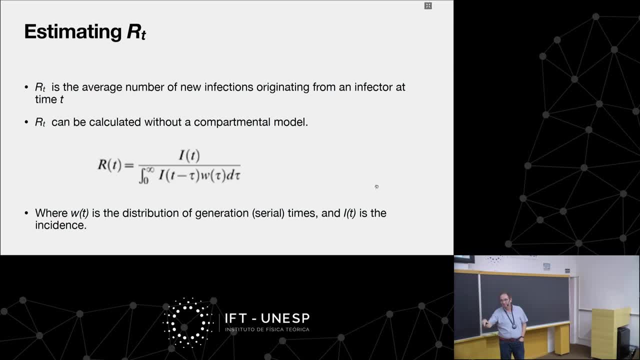 incidence, the number of new cases per day- okay, number of new cases per day- and which is something you know, okay, for instance, when you look at SIR model, you don't know less usually because you don't know, I I the number of people that are infected at that at a certain moment of time. you. 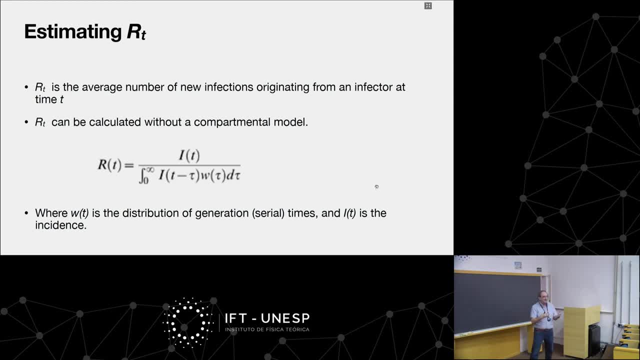 don't know this. usually what you know is truly, notification system, how many new cases you have per day. okay, so the number of new cases per day, it's, it's the kind of of data that exists, and and then you have to know which is something. this. 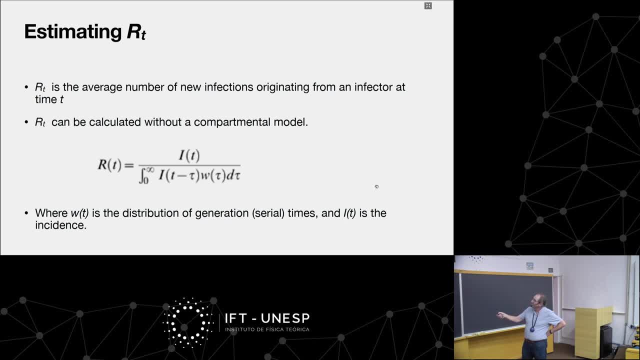 is this W, which is the distribution of serial time. serial time is the following: say I, I am, I just got infected. okay, better, I got my first symptoms and then I infect somebody and this person will have the first sentence on some days later. so this time between the first sentence of one person, so the other person is called. 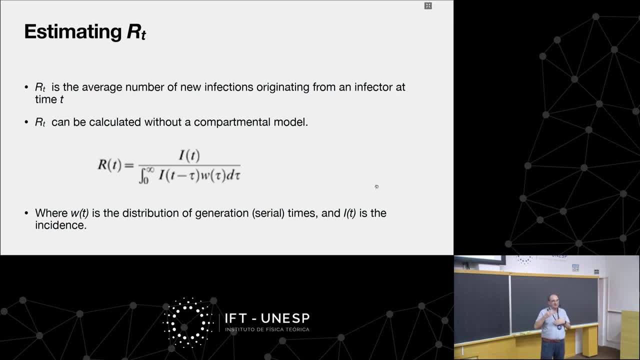 the serial time right and there is a distribution, but it's not everybody has the same exactly, it's not okay. so there's a distribution of serial time. so So, knowing this, you can calculate R of t. Nice, It seems. everything is just fine. 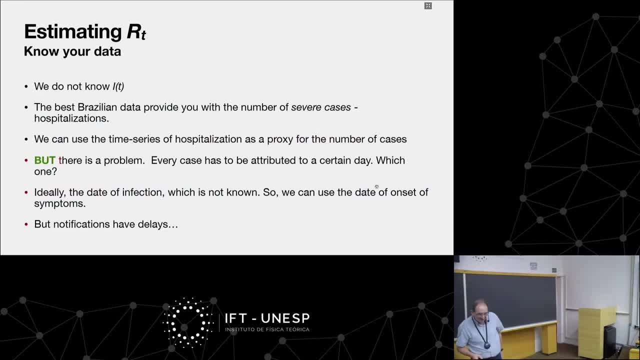 But well, things turned out to be much more complicated because, well, now you are interested in an epidemic that is just going on, like COVID. It's not the past epidemic, So you have a problem with your data. You don't know, actually. I. 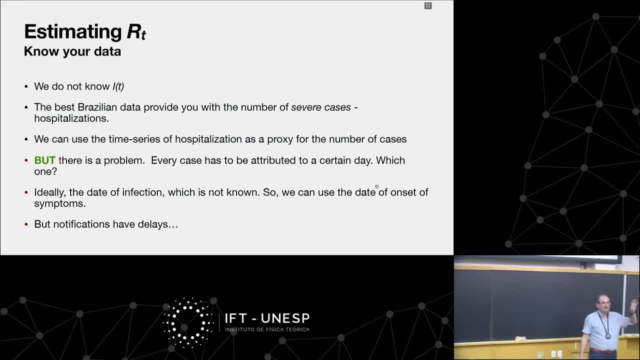 In Brazil. what you know is the number of severe cases. so you have the I for the severe cases, okay, Which you can think it's a proxy of the total number. It's reasonable, Okay, but then you have a problem. 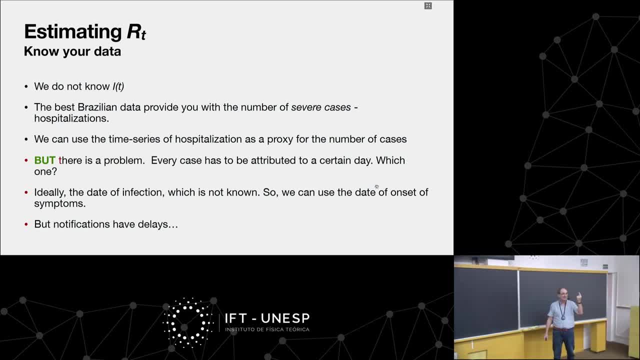 which is, every case has to have a date in order to have number of new cases Today, so every day. So every case has a date. What is the date of the case? So the first thing is: people announce, usually government announces. 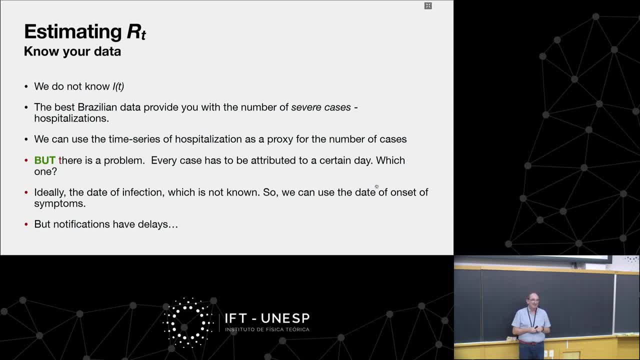 number of new cases have been notified today. okay, This is not epidemic parameter, epidemic variable, It's an administrative. depends on the notification system. Okay, They can take. in Brazil, there are places it takes three weeks to notify one case. 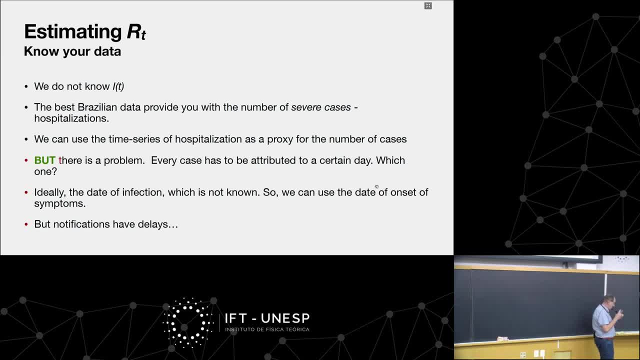 So you should actually do something. better is you should connect one case with the date of first symptoms. Actually, you would like to connect it with the date of infection, but nobody knows exactly when it was infected. but people know the date of first symptoms. Okay, So then you should report it to the date of first symptoms, which is in the database of COVID cases. It is, It is, But notifications have delays, and so you have to have the notification to know the date of first symptoms. 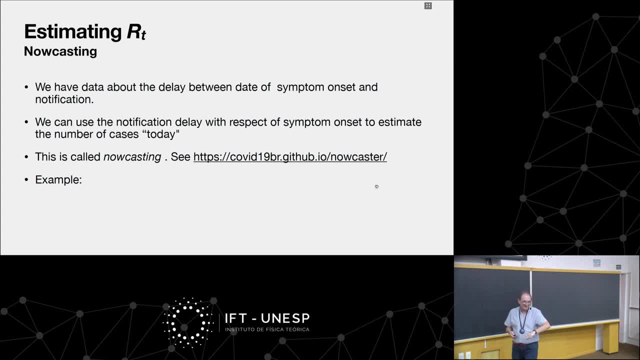 Okay, So you are always late, So you have this delay between the symptom onset and the notification. Okay, So what you have to do is use statistical- it's usually Bayesian- analysis and so on, and I'm not really a specialist on this. 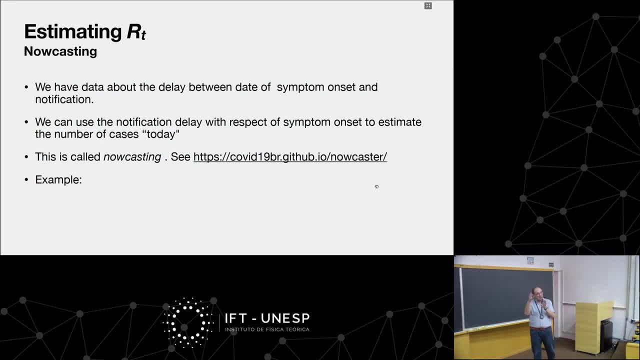 but knowing the distribution of delays between onset of symptoms and notification, and having some notifications going on already, you can estimate the number of new cases today, which is called nowcasting, which is a kind of joke with forecasting, but it's not, for, it's just now. 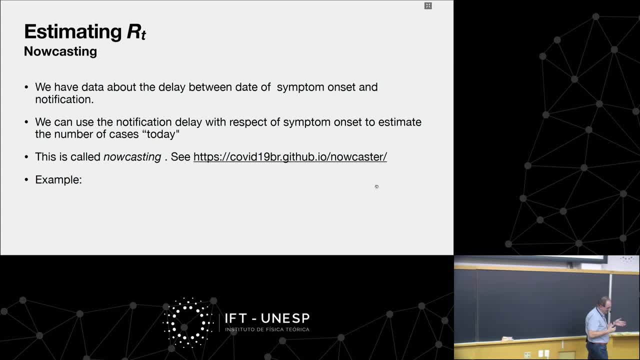 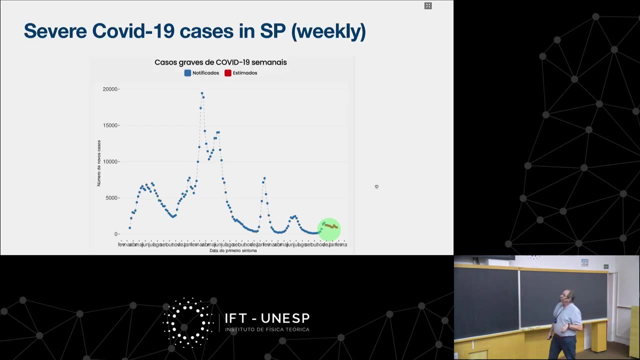 Okay, So you actually it's not so much now, it's like five days ago, And so you have to first do the nowcasting and then calculate RT over the nowcasted things. Okay, So if you look at, this is a plot from. 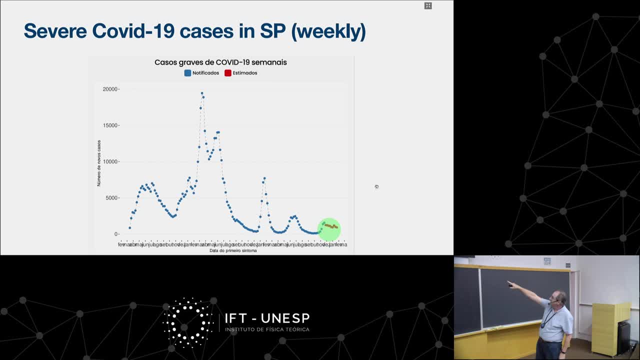 again from St Paul and you see that there is some data which was in red. These are nowcasted data. If you look at the data, at the raw data, there's just a sudden jump going almost to zero, which is not real. 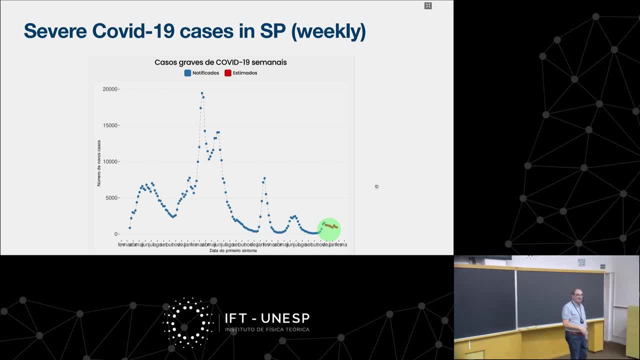 It's just the fact that there are delays, So you estimate this and so you have to do this nowcasting. So this is something important. if you are modeling for outbreaks that are taking place now, Okay, If it's in the past, all data is consolidated. 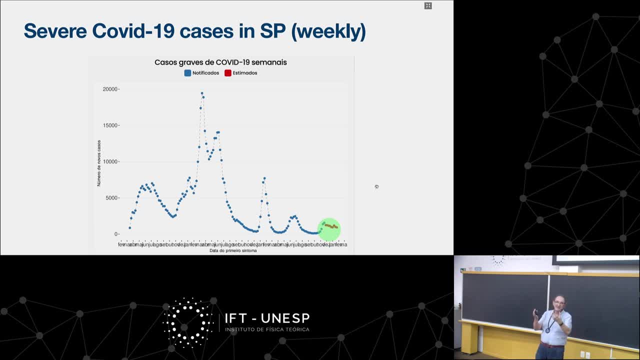 you don't need anything of this, But if it's outbreak, you need it now And you have these delays and you have to go through statistical methods to estimate how many cases you have. I have a question. Yeah, These red dots are estimates. 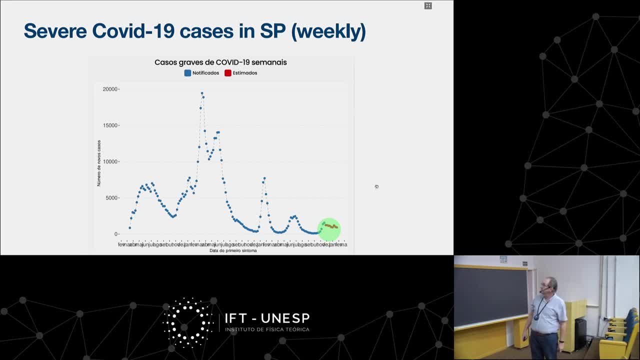 But when I compare this part of the curve with the, say, the second peak from this point behind, I don't see this plateau. I see this going downwards Right, Fast. Yeah, This was the estimate. I don't know what. 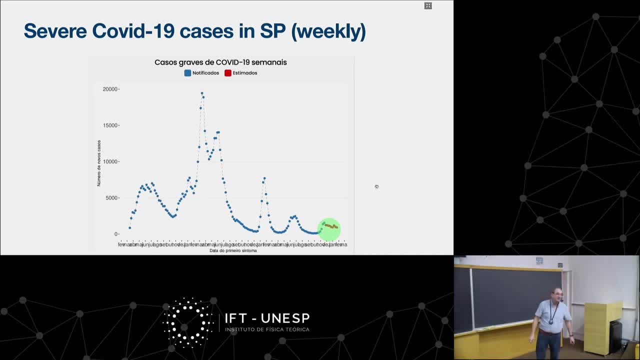 So, okay, What I mean is we are predicting somehow a different decay in comparison to previous ones. I didn't show you the credibility interval. What? Sorry, There's a credibility interval. There are errors around. Okay, This is just the. 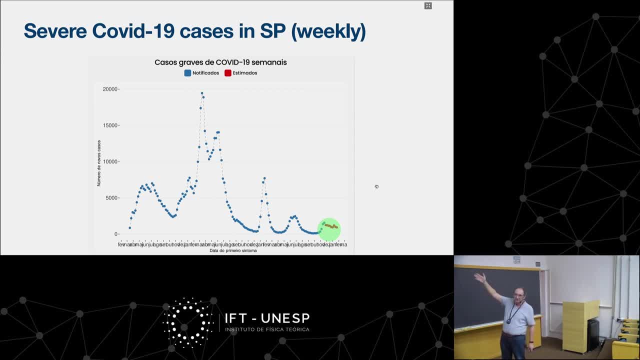 The. That's something that we actually A site that we built for a large public. Okay, So there are error bars and so on. You obviously tested if our Using the past, if our null casting is okay, There has been validation before. 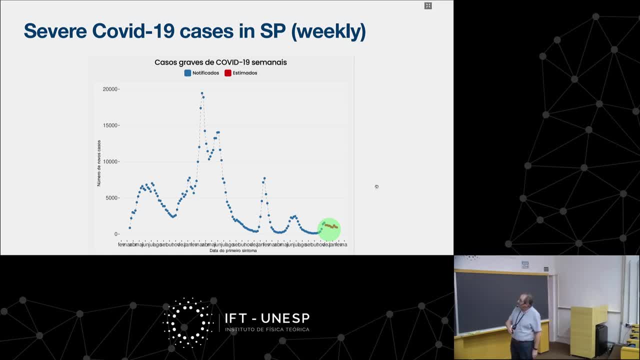 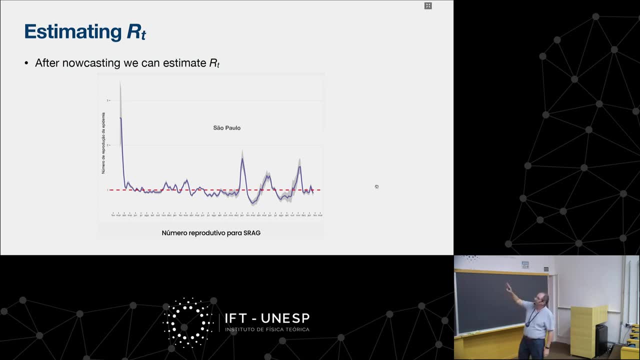 Okay, So once you have this, then you can calculate RT. This is a typical thing that you have, For instance, for Sao Paulo. it is always The line: is R equal to one and has been bumping up and down around. 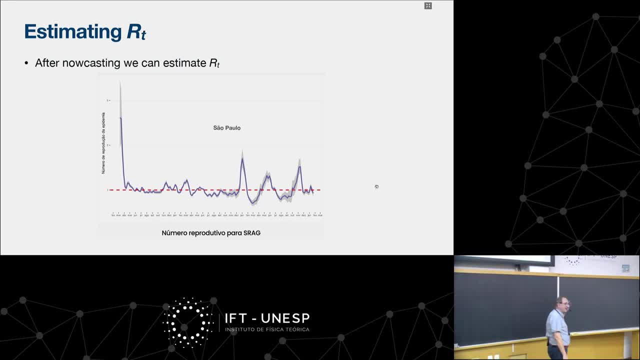 So it can increase because usually we had variance and so on. This is from the beginning until March. Until this, I think this is February, February 21,, 22.. Yeah, But the beginning of 23 until January February. 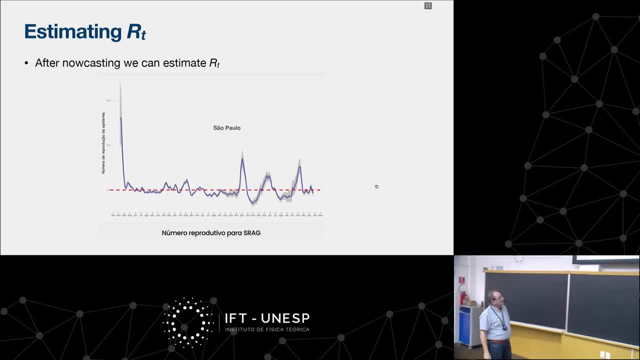 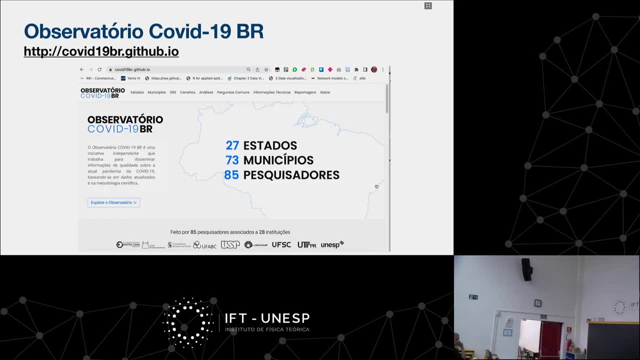 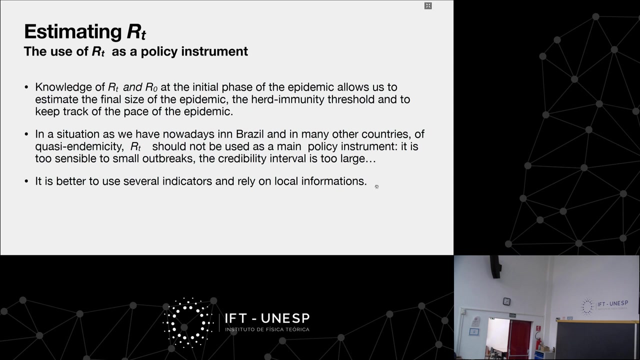 Yeah, there had some small bump. So now let me comment on this because, okay, So this is our site, if you are interested. It's called Observatory COVID with Nazari Berger And so. So the point about this RT: you cannot use it blindly because when you are at the very beginning you have a lot of susceptibles and so on. so knowing R, R0 or RT at the beginning it's important because you can estimate how dangerous this can be, actually because it's connected to the final size. 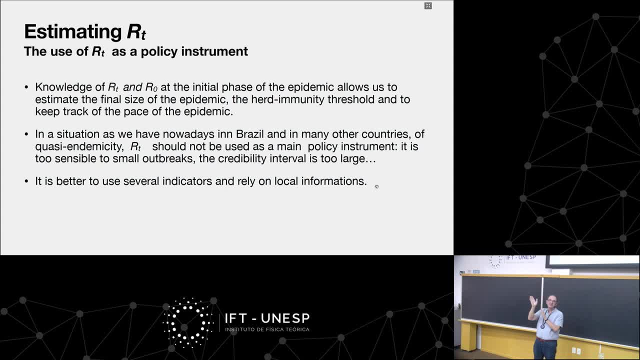 And you can keep on the progress of the epidemic by looking at RT. but once you are back to some very low level of infections, then sometimes a small outbreak will get you an RT bigger than one and therefore you should have more and this should not trigger an alarm saying: 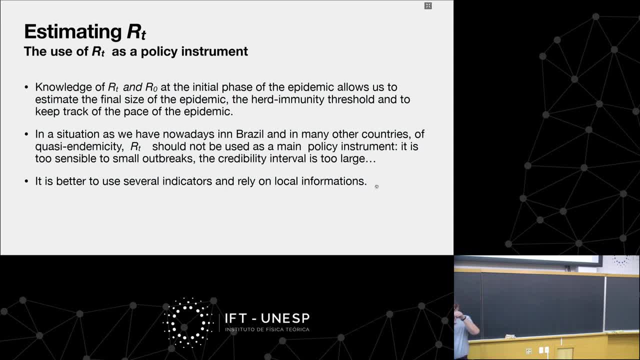 everybody has to stay at home and so on, because it's localised. but as the baseline is a very small number, any small outbreak in some place will give you an RT. So RT is an interesting parameter to use for decision making about epidemics, but not necessarily it is this only parameter. 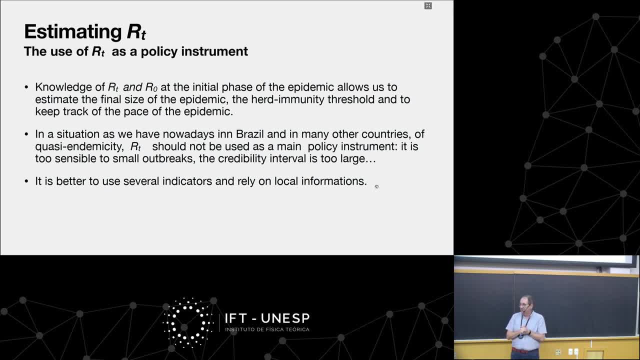 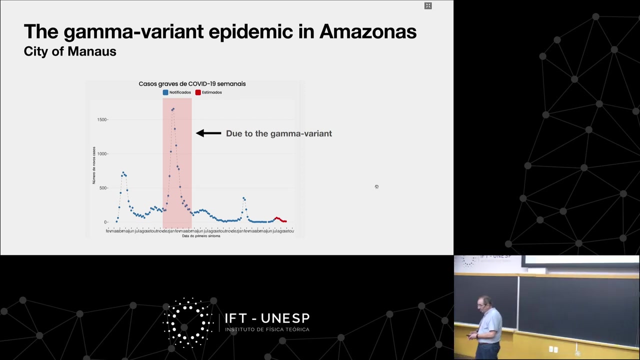 it has to be part of a bigger set of parameters, A set of parameters that can actually evaluate the best actions at a certain point of time. So let me just give the second example, which is about the cases of COVID-19 in the city of Manaus. 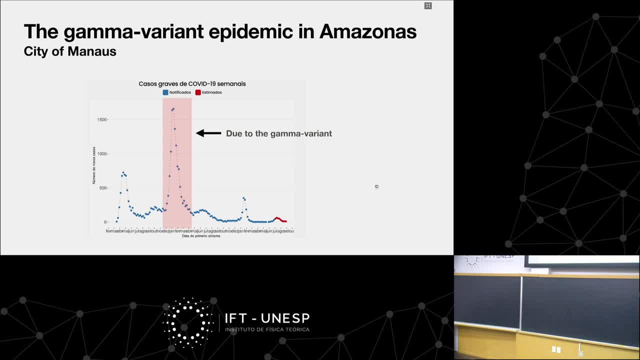 at the beginning of the pandemic In the beginning of 2021, which has been known as a very catastrophic situation and there has been a discussion about- because Manaus had already had lots of cases before and there was an estimate that 78% of the population had COVID. 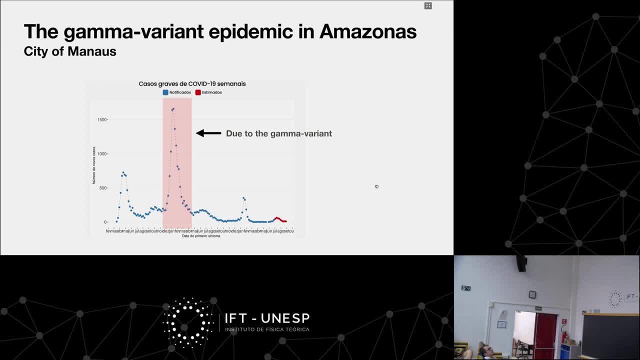 In October. So you're going to say, well, it will be difficult to have a new epidemic there because there are so many immune people. But what we didn't know in 2020 was about waning immunity. Immunity doesn't stay for a long time and if you have variants, sometimes you are not immune at all. 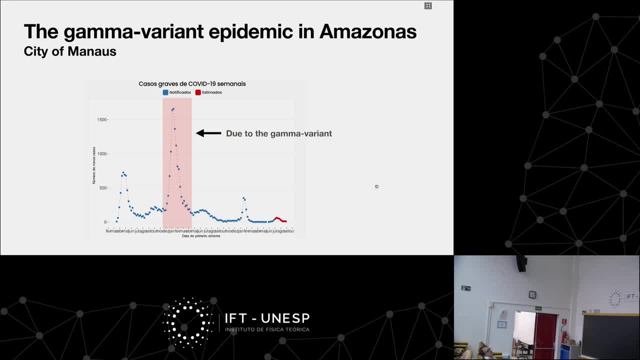 So this was not known. So there had been a very big discussion about this result of 78%, which was based on examining COVID infections with blood donors, And so what we know now is that there was a new variant, which is what's called the P1, and then gamma variant, and so on. 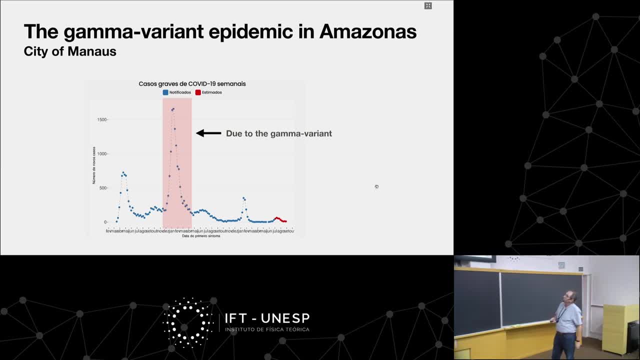 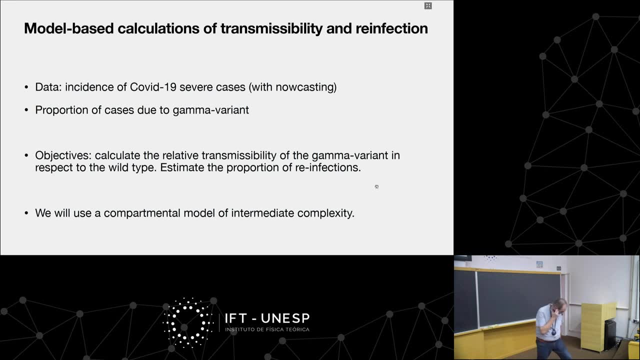 which was responsible for this super high peak and all the catastrophic things that we had. And so what we did is we worked on a model which has the wild, the resident variant, and the gamma variant, which is the invading variant, And, in order to estimate, 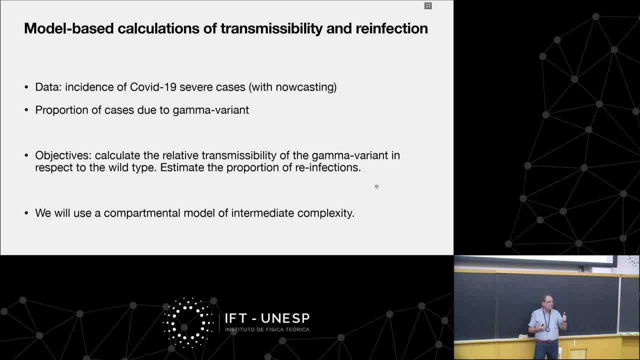 two things. One is how many times is the gamma variant more infectious than the wild one, And how many reinfection cases can be attributed to the gamma variant. So these are things that we wanted to know. So what we had is the incidence, the number of new cases per day. 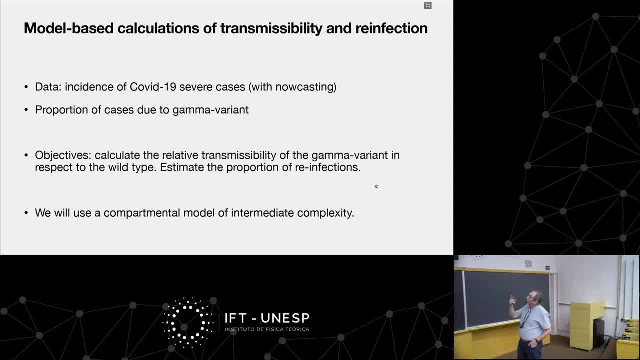 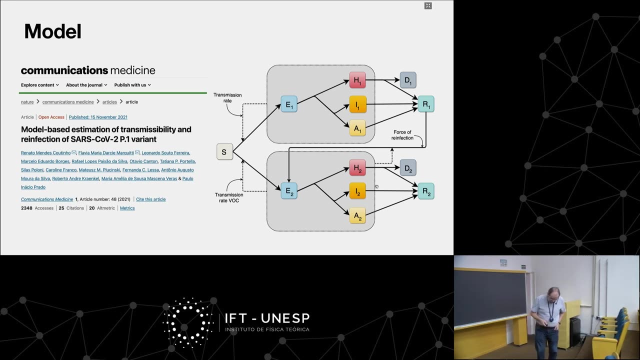 For COVID-19. And the proportion of cases due to the gamma variant. Because there are people that were doing surveillance, genomic surveillance, at that time, So we were out on. we have a model which we call the medium complexity model. 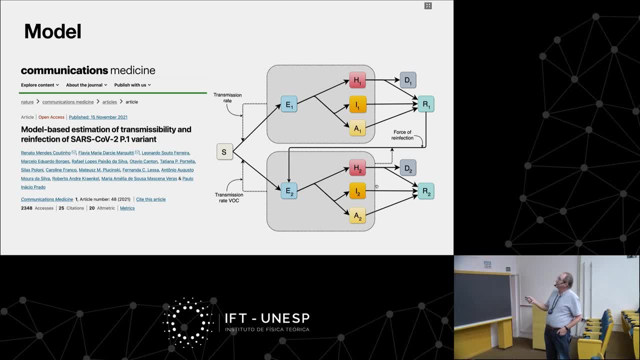 which you have the susceptibles, and you have here a compartment for the variant which is the resident variant And this is the invading. This is gamma And after being exposed people can get to the hospital, get asymptomatic or just have symptoms. 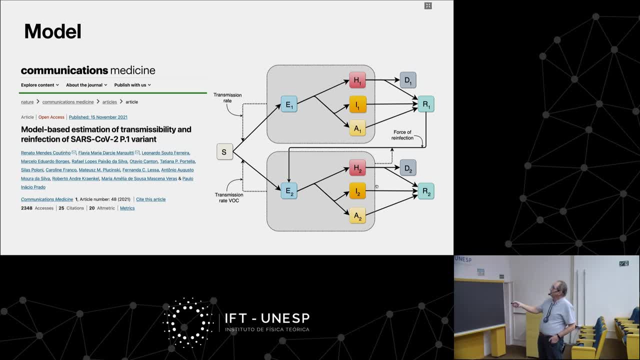 but not go to the hospital. Both cases are the same. Then now some of them. we suppose that the deaths are only related to the hospitalized cases. Then you can get recovered, recovered, But the recovered from one can get infected by the second one. 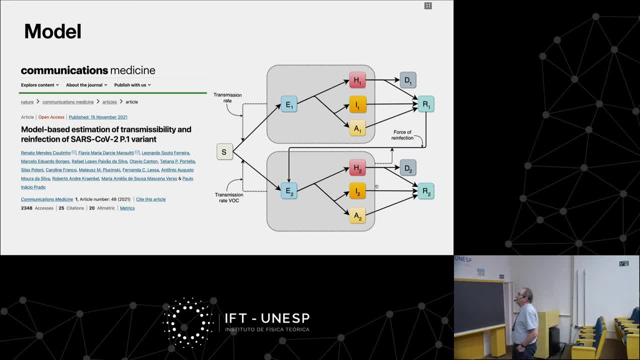 Okay, So, and then all of this is divided in three age classes: From zero to 20, from 20 to 60 and over 60. Because mortality is strongly dependent on ages. So you do this and then you do data fitting and a lot of things. 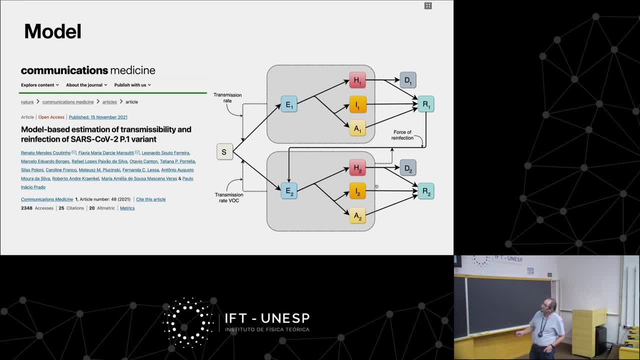 And you see that the number of authors starts to increase. There's many different things you have to know And people that do the fitting people that know more about epidemiology, and so on, And so what we found with this, come on, okay. 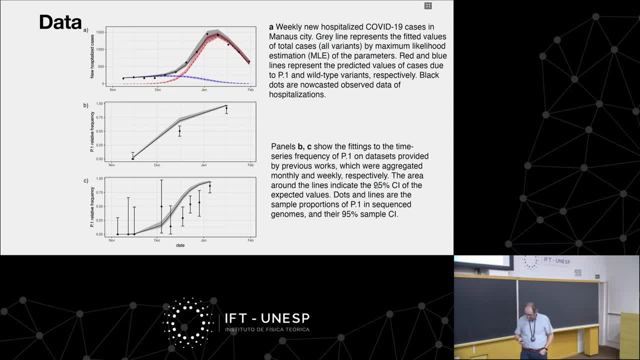 So the data we had was actually the epidemic curve. The epidemic curve, which are the black dots And this shadow? here is what our model predicts. And then you have also the number of wild, the proportion of wild cases to the gamma variant cases. 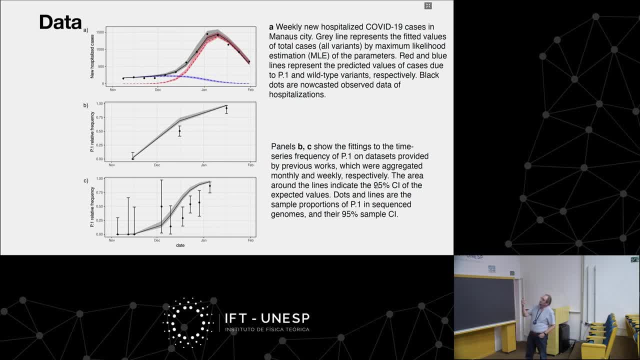 Here. this is the proportions, So this is the data that you actually have And you go for fitting and so on, And I don't want to take much time about this. And, come on, Sorry, Roberto, What's calculated and what are data? 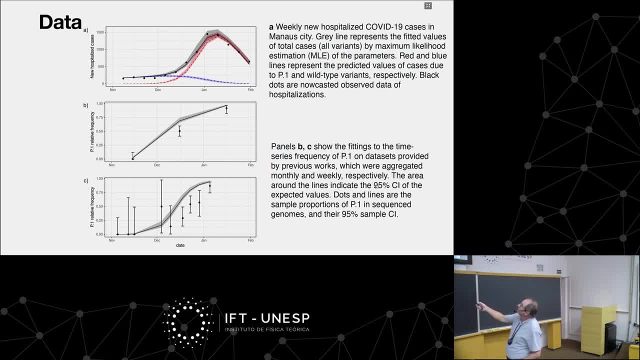 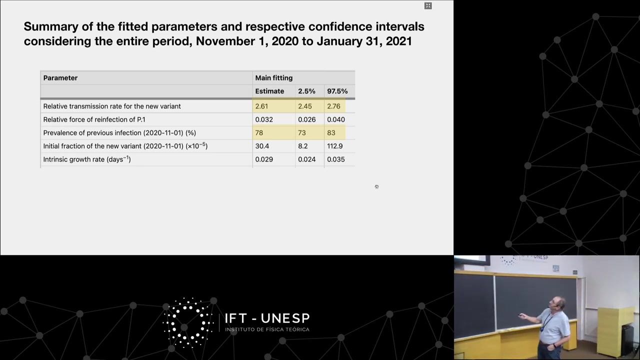 Data: are the dots Okay And the calculated? is this Okay, This strip here And okay. So I think I have time, Let's go over this here. So these are the results. But what is important for us here is that the relative transmission rate for the new variant is 2.6 times the transmission rate for the old variant. 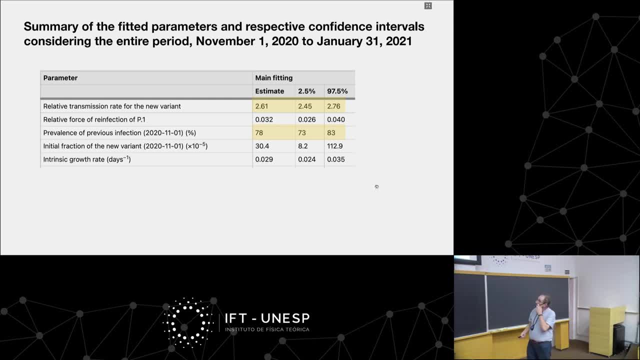 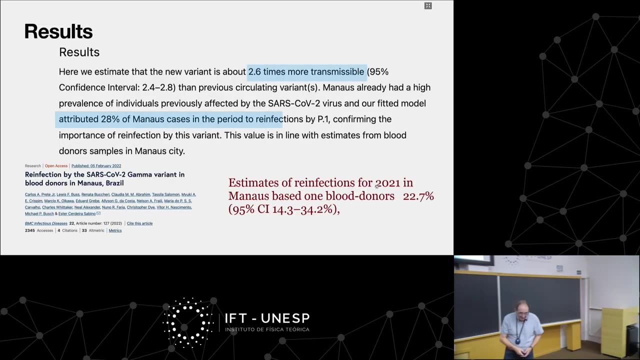 Okay, So it's relative. Okay, So it's much more infectious, Much more Okay, 2.6 times. And then they have the credibility intervals and so on. And well, what is nice that from this you can calculate also the number of estimated reinfections. 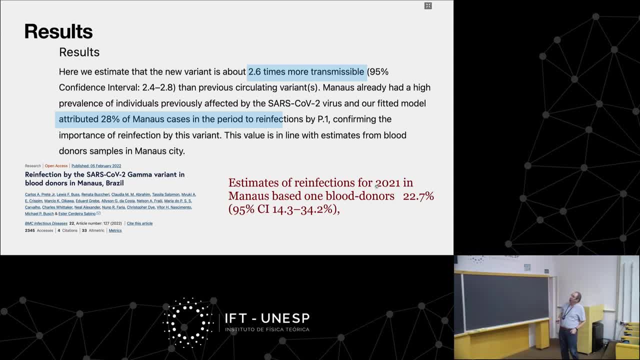 And what we calculated is that 28% of the Manaus cases in the period which goes from 1st November until 31st January, which is the data we used, 28% of the cases were reinfections. So you have to have reinfections in order to understand what happened in Manaus. 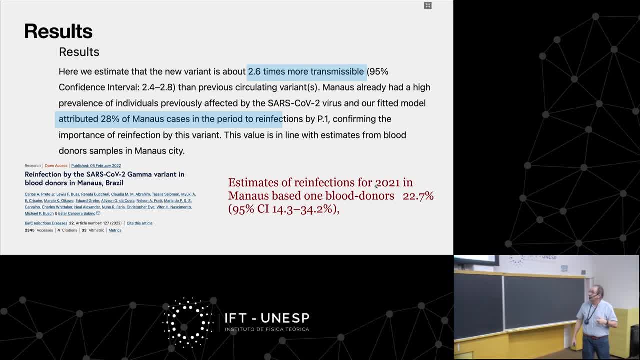 Okay, And actually one thing that we also calculated is that which was a free parameter was the number of people that already were immune to the wild variant at the beginning of November, And actually we got the 78% that people had shown to, I mean had estimated from blood donors. 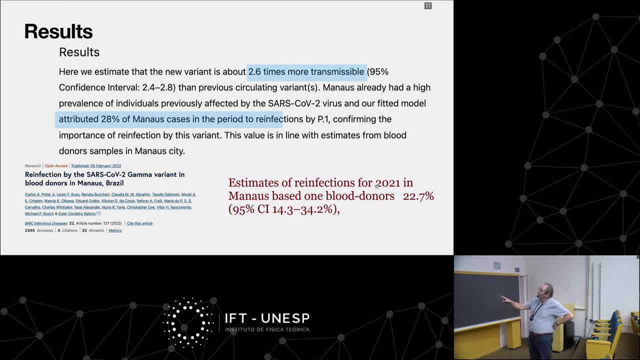 And so this 28%. then actually there has been people again working with blood donors, which is the group of Esther Sabino from USP, and actually went on to calculate how many reinfections they have. This was estimated later. 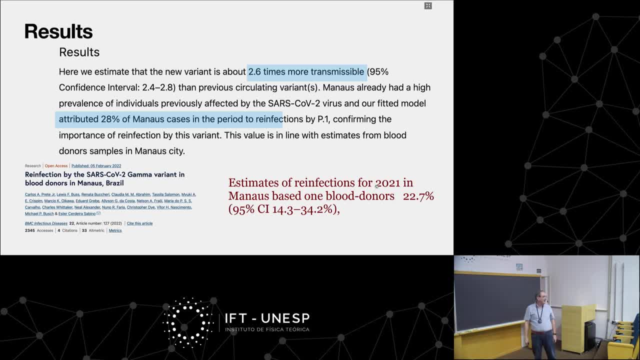 And actually our results are okay with that. So the explanation for what happened in Manaus is this: Okay, So this is a combination of reinfections and highly transmissible strain variant. So that's one explanation, Yeah. 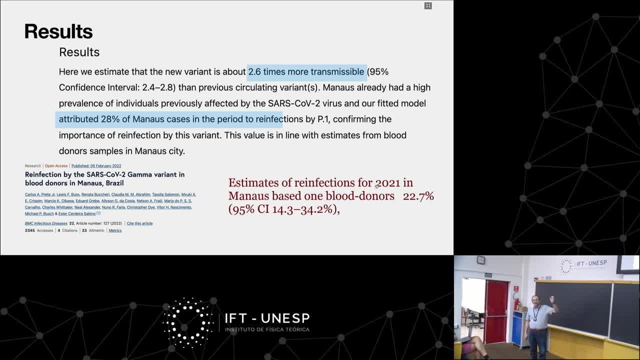 I mean it is in principle. well, this one with gamma variant It's not comparable, because I mean it would be comparable to other cities in Brazil, No, no, Outside other places in the world. Yeah, But gamma was essentially here. 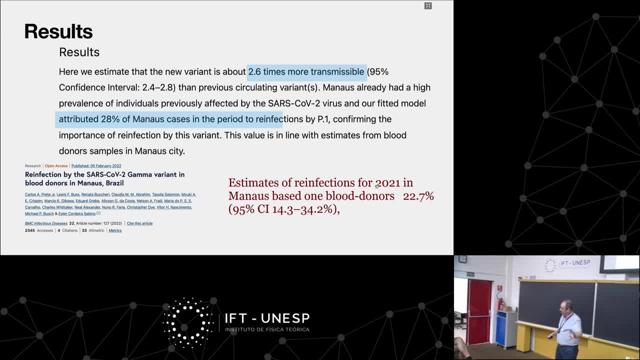 Okay, It was only in Brazil, Okay, And something a little bit in Argentina, Peru and so on, But gamma did. it was a very important, and something that we don't understand is why didn't gamma go to the world? 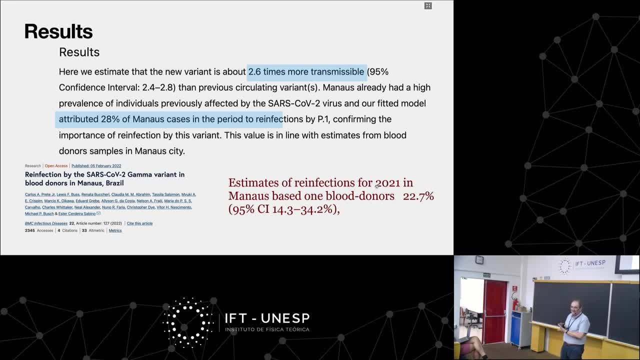 That's something we don't understand. Okay, Probably at the same time that gamma was increasing here you had delta in Europe And maybe there's kind of competition between them. Okay, But for instance, people in UK, they estimated this kind of things for delta variant. 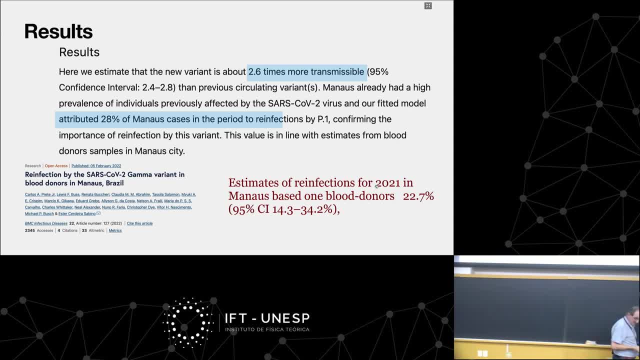 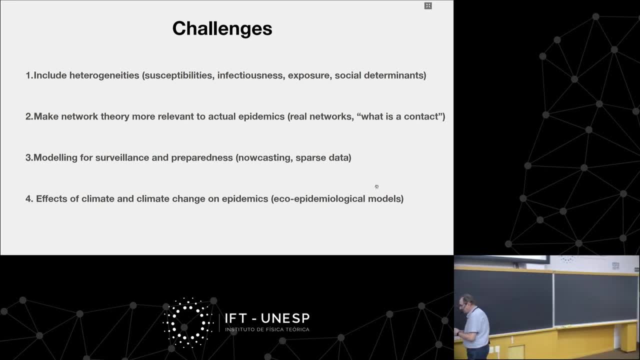 Okay, Okay. So these are the examples, And let me now just finish by talking about some of the perspectives in the area of mathematical modeling and epidemiology. So let me state some of the problems that are difficult today. So one is having included in your models the fact that populations of people, or even 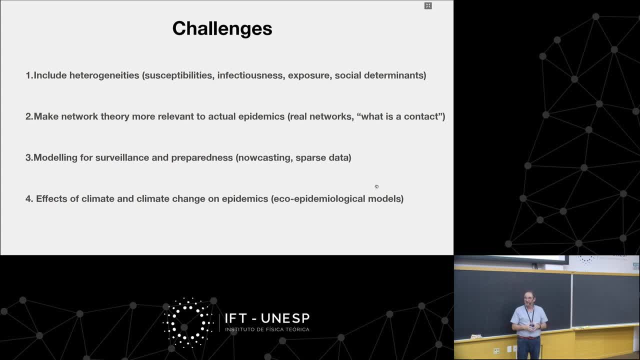 for vector-borne also, mosquitoes and so on, are heterogeneous. Heterogeneous in which sense That people have different, Have different susceptibilities. Susceptibility is how easy you get the disease And have different infectivities how easily you transmit the disease. 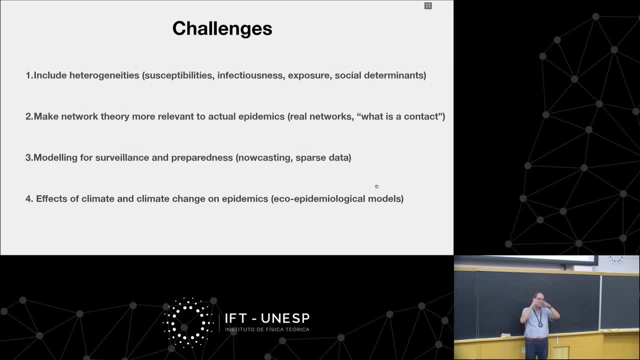 So there are people that, due to the immune system, there are many things that have more propensity to either to infect or to be infected. Therefore, this will impact this parameter that was the beta, which is the probability of actually getting, In fact, if susceptible meets an infected person. 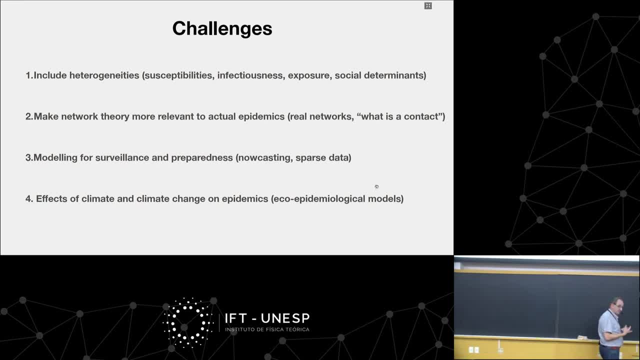 This beta should actually be a distribution. Okay, So there's not. This should take into account the fact that people are different and you cannot necessarily take the average infectivity and susceptibility. There are important effects that can come from the fact that there's actually a distribution. 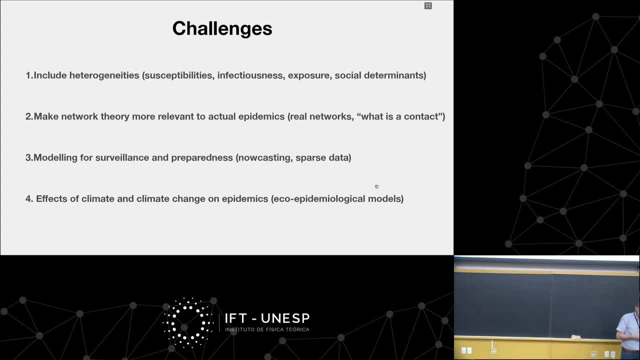 of susceptibility and infectiousness, And also one of the important things is different exposures. So, for instance, exposure is very important for dengue or malaria, Because when you do models, one thing is you have to know which is the population at risk. 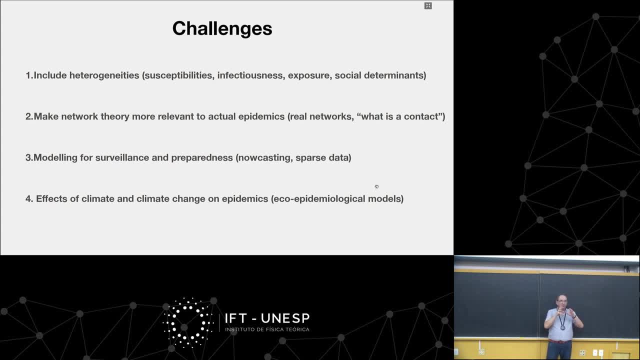 Because it's. What's the total population? Is it the population of the city or of the country or whatever? What are you modeling? Okay, So if a population is not at risk, it should not be taken into account in the model. 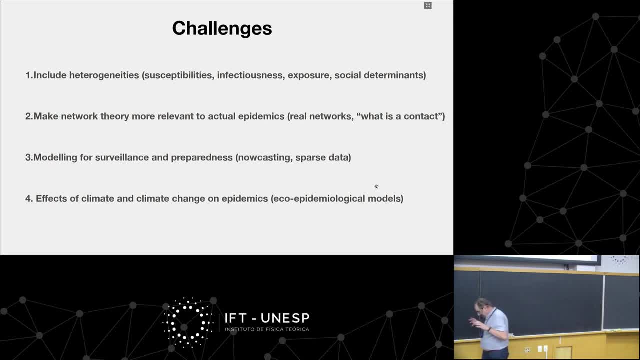 Okay So, but even if you look at the level of a city, there are places where you have more exposure than others, And this is typical for vector borne, for insects. Okay So, this is the heterogeneities, which are spatial heterogeneities, which are usually. 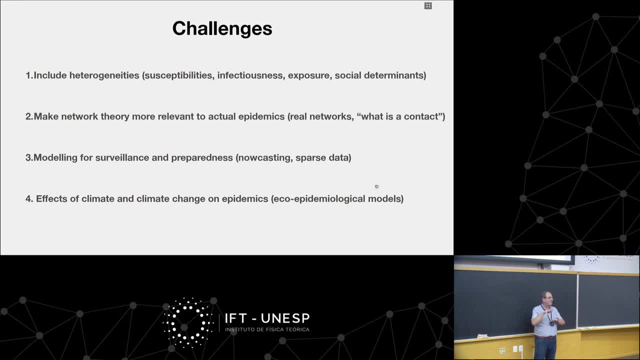 connected also to social determinants. People having access to clear water or sanitation, And also social determinants are important for mortality- Having access to medical facilities or not. Okay, So all of this is heterogeneous, It's not constant, And the first approximation of all the models is to take it constant. 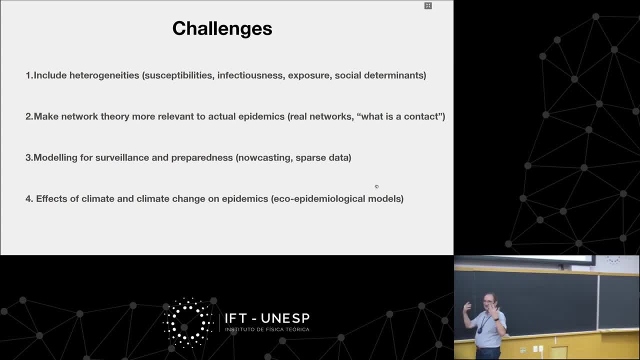 But actually you should take this as some kind of distributions, Okay, So another thing which is important is the use of network theory. Network theory has been kind of wiped for some time. So how are networks used in epidemiology? Most of the time, each node of a network is a person. 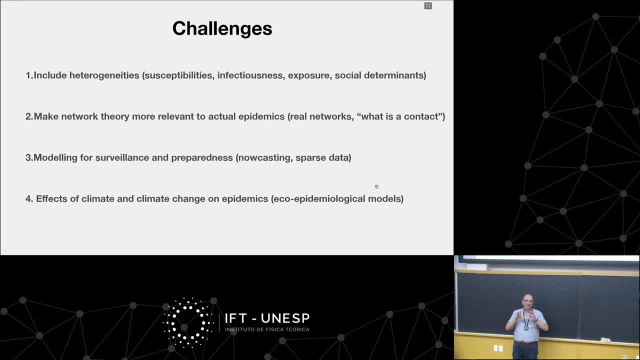 And you connect persons if they have contact And then you have a network of contacts And then you have the epidemic dynamics on that network And what This has been studied over 20 years ago. Maybe you have non-trivial networks. Non-trivial networks is kind of a network of people that are interested. 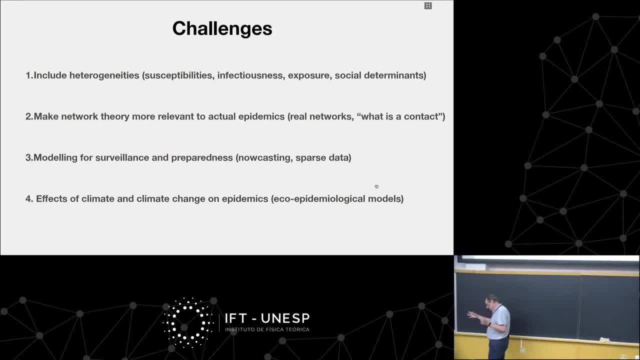 For a network. the number of connections I have is my degree, So you have a degree distribution Okay In the network And usually in a random network and so on. this will decay very fast for large degrees. But then what happens? 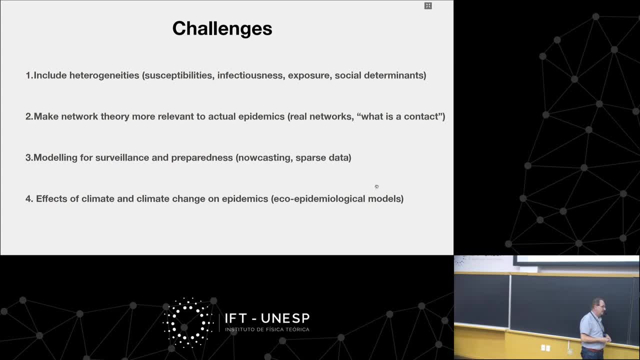 But then sometimes you have structures in the network which make it have a long tail, So the decay is polynomial sometimes Instead of being exponential. This is the kind of thing that people have studied a lot with networks in general and also in the epidemic. 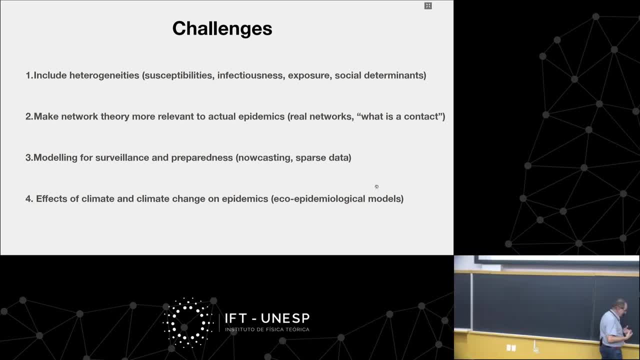 And then suddenly the structure of the network has importance about the parameters of your equation. For instance, calculating the beta has some influence from the structure of the network of contacts. So this has been explored pretty much Very nice results. For instance, if you have this kind of degree distribution with a fat tail. 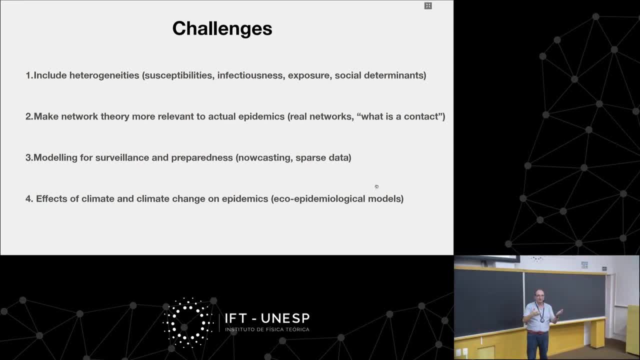 then it's much easier for a pathogen to invade because you have superspreaders, But actually the total size may be smaller than in the case of random things. So there are interesting cases And maybe this can be very important And sometimes, if I 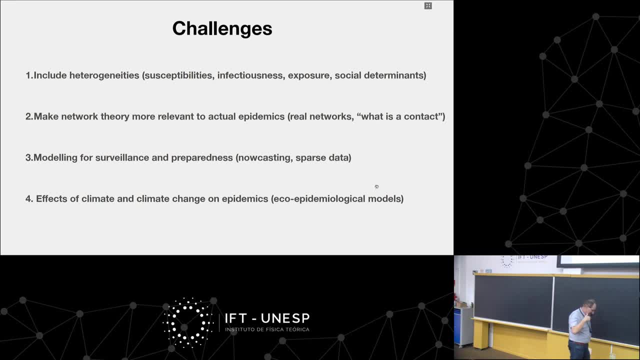 I don't have so much time, but I could speak at the end about mpox- Monkeypox, Which is connected, probably, to a problem with degree distribution of contacts, But the point is, most of the time people do this and do not connect this to any data. 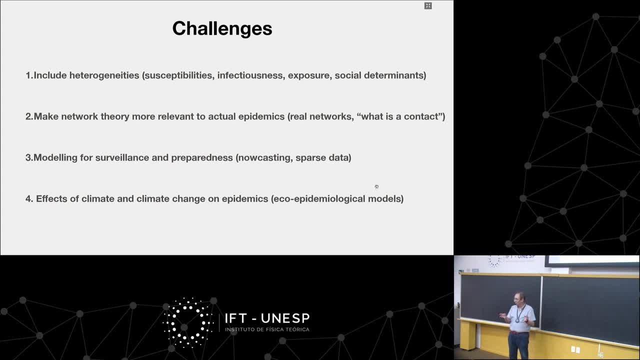 It's nice to publish in physical review, But what's the importance of this in actually explaining some epidemiological facts? So the first thing, which is very difficult, is: Okay, we have a network And then go for an epidemiologist to say: 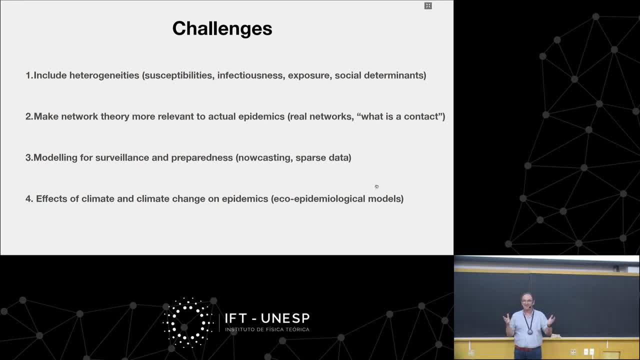 What You have, a network? I don't have networks. People don't know things about contacts. Okay, So it is for us. we think about networks as something that can be given. But then there are two questions, two points. 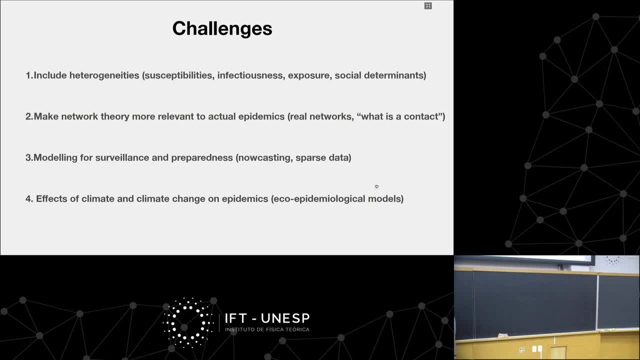 First, what is contact Okay For respiratory diseases? What is contact? I'm in contact with you or not? Okay, How long is my contact? Is everybody in contact or not? So what's contact Okay? So that's already a problem. 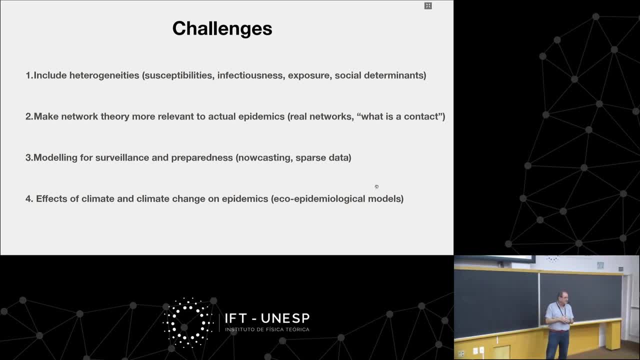 Okay, Depends on the way I mean the transmission type, One place where contact is defined for sexually transmitted diseases. it's a classical thing. But then you have a different problem: How do you know the network? Well, you can't say I'm naive and I go and ask people. 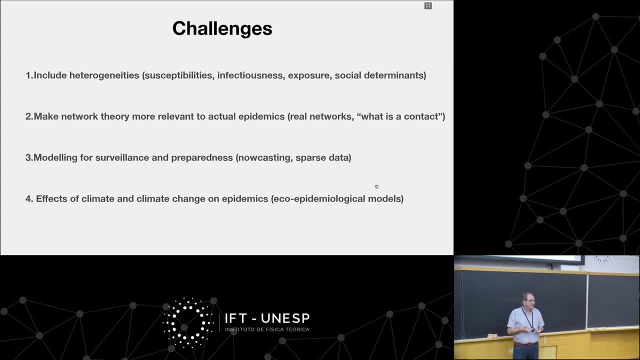 Okay, But you know people lie And especially related to sexual things, So it is not easy to know a network of people that had partners. Okay, And there are special. There's a Part of epidemiology that's called field epidemiology, which is about how you access. 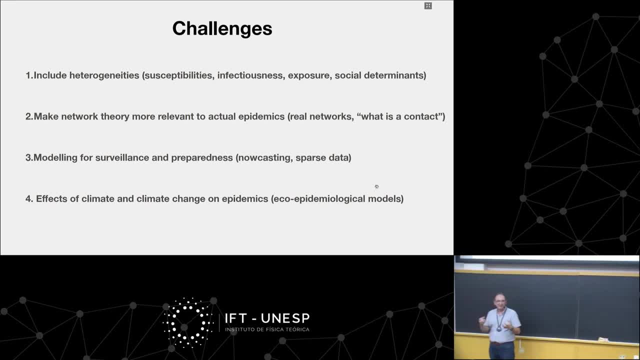 actually this kind of data, Okay, How you know who had contact, for instance, And you use some techniques which is called pair navigation, which is the people that will actually do interviews, are people that are also from the population that this is. 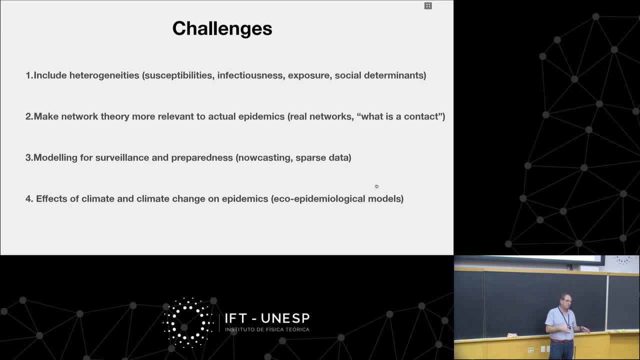 the object. Okay, For instance, if you were working with, for instance, transsexual people, Then the people that do the interviews are also transsexual, So it creates trust, for instance. So yeah, there's a lot of things like this. 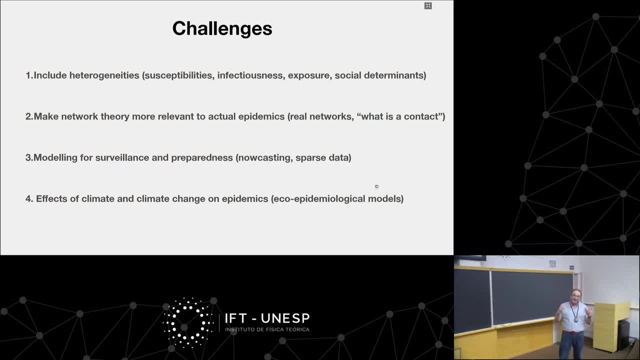 And in obtaining this kind of networks it's actually very difficult. What is easier to obtain is the degree distribution. People more or less will say: I had so many partners last year. Okay, This is better. But when you ask them to name the partners, 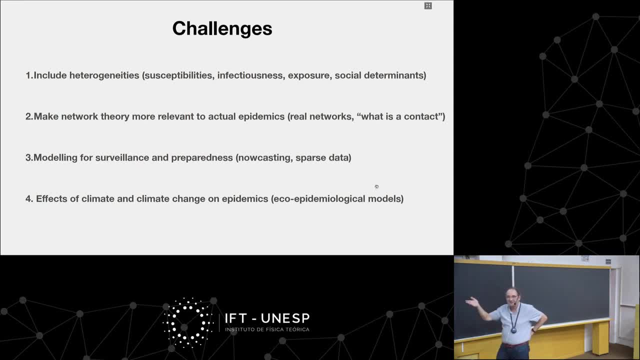 Then you have a problem. People don't want to, They don't know you, And they say I won't give you this data. Okay, So one point is connecting network theory to real networks. It's not easy And this is still a challenge. 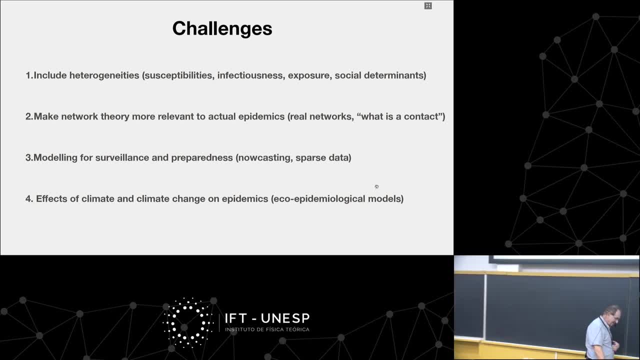 And well then there's this kind of thing that we have been going through with COVID-19.. And then it's the modeling for surveillance and preparedness. So one thing is, for instance, looking at historical epidemics and looking if models 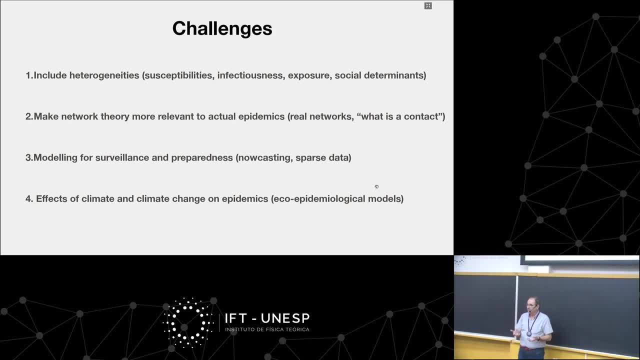 can help you understand better what happened, and so on. But sometimes you have the situation that you have just an outbreak of something new, for instance like COVID-19 or something that can happen, And then you should have ways of doing Contributing using modeling. 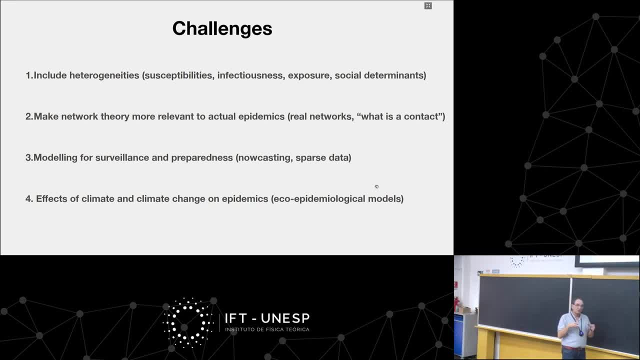 Mainly also statistical analysis to assess the situation, which is different than models that look at historic epidemics, And this needs the kind of things like now- testing and other techniques from sampling and statistical sampling in order to access the situation of an outbreak at the beginning. 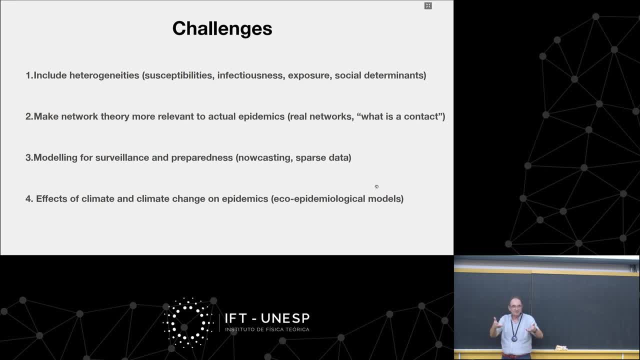 of something. Is it dangerous? Is it not dangerous? How worse? How Can it be very bad or not? So you have sparse data and have a lot of problems. So you have to try to integrate different sources of data. 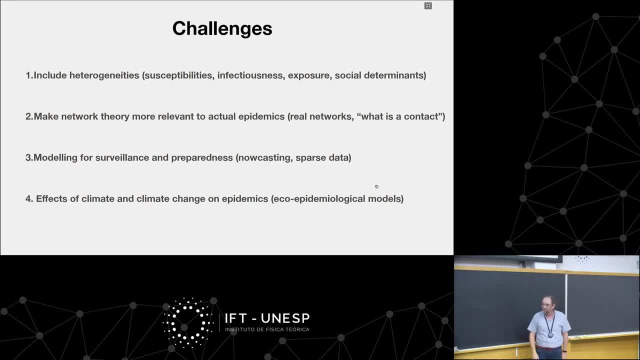 Sometimes you use Google searches or something in order to access the situation. And finally, one interesting thing is also climate change and diseases, But this is very important usually for diseases that are transmitted. They are transmitted by animals, by insects, for instance. 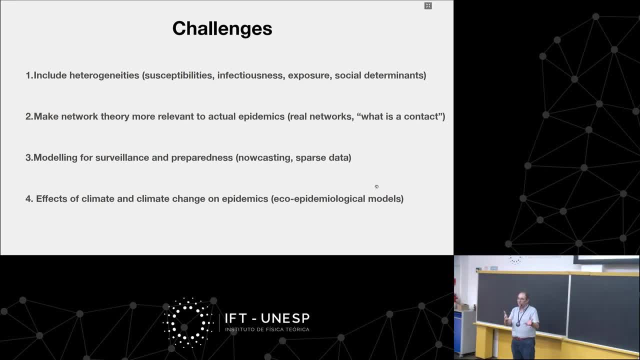 Insects, which are insect-borne diseases like dengue, malaria, yellow fever and so on They have. They are related to climate change in a very important way, because these insects do not regulate temperature. If they have a temperature difference, then all the metabolism of these insects will be. 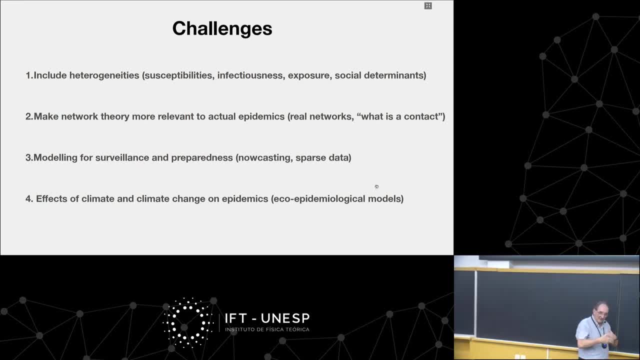 different. If it's hotter, then they have a faster metabolism, and so on. So this in fact affects everything And actually there have been studies which try to model which is not the population of insects but, just to say, is a population viable in a certain place with certain meteorological. 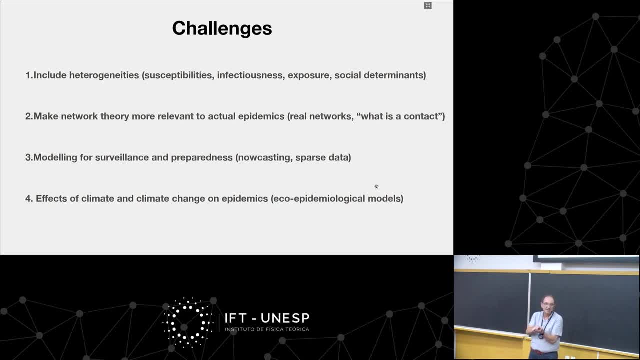 conditions or climatic conditions, And then use these big models of climate change and say: well, will the certain population of certain insects, will it be shifting the range of occurrence or not? in which direction, and how can this affect the contact of this population of insects with other animals? or 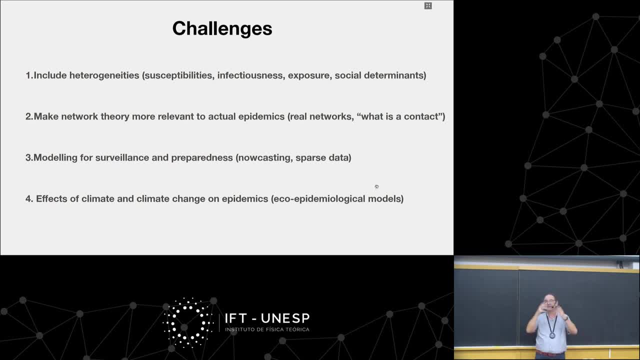 with human beings. So this is typically a very important thing. So this is a very important thing. So this is typically a highly computational task because integrating all the climatic models, which are super big models, and so on, but this is also one challenge to model. 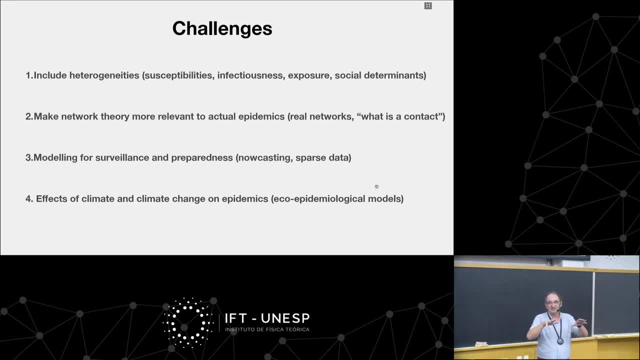 what could be the effects of changing climate in the occurrence of diseases. So one example is- I mean this has not been fully discussed and that's one thing that we are actually in our group discussing, which is, for instance, the range of occurrence of dengue has been 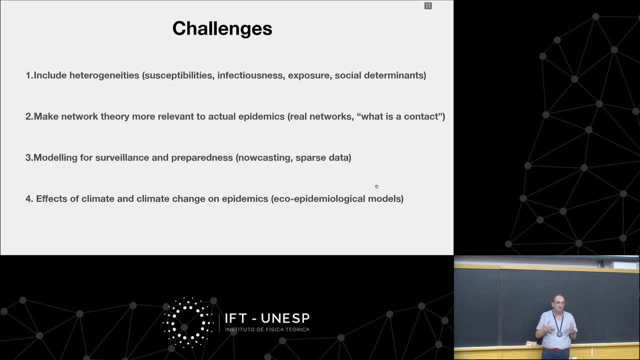 shifting south in Brazil. You didn't have dengue in Porto Alegre for 10 years ago- 15 years ago- and now you have. It's very curious because you don't have every year, So there is the possibility to have. 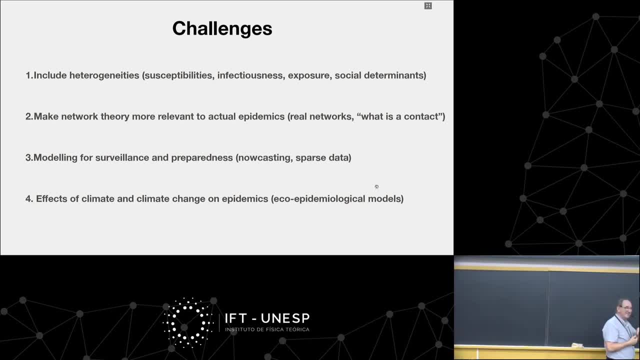 But you have every year. you have the insects, But some years you don't have the epidemic on the insects. So what is happening? So that's kind of the region which is the fringe between occurrence and non-occurrence of the disease and also occurrence or non-occurrence of the insects. 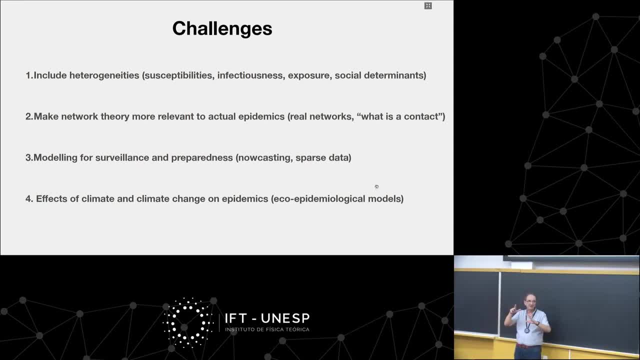 And this can be affected by climate change or by land use change, also the different things, not only climate change. So what is going on? Is it going really south? You have Now you have dengue and Buenos Aires also, which you didn't right. 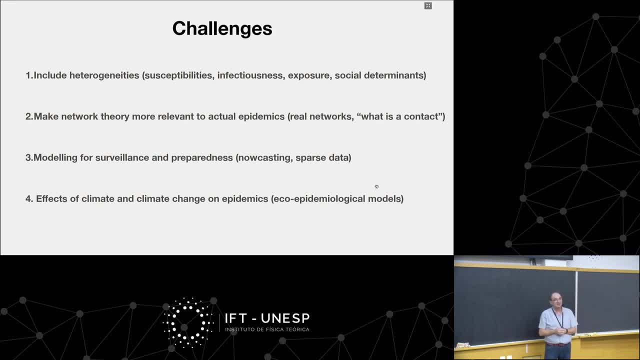 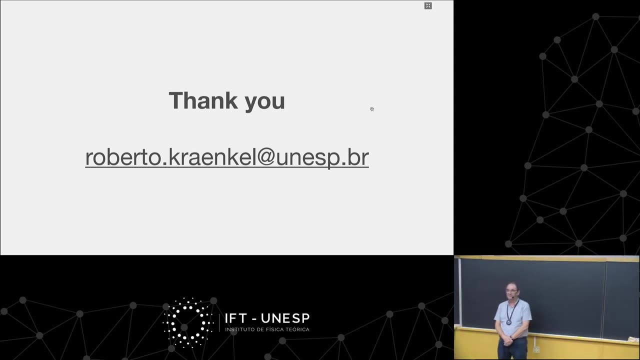 So there is a shift and understanding this is still a change. So, okay, Thank you. That's all for me. Thank you, Roberto, So we have some time for questions. There are many hands raised. Go ahead. 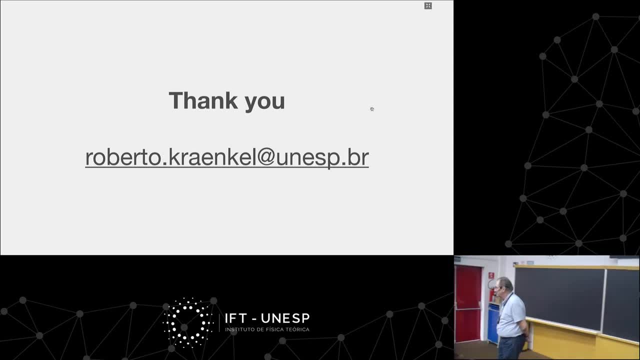 So from your talk, it looks like most of the challenges are for social science. It's not really mathematical challenges, Is that correct? Well, yeah, It is to a certain extent. There are mathematical challenges with networks. still okay, because you have to look at networks. 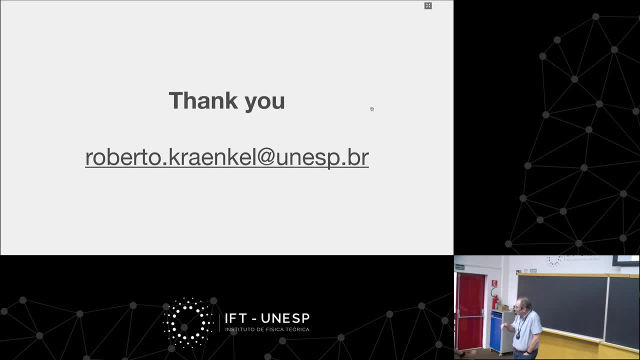 that have time dependence in the connections and this is not well studied. okay, But yes, And many challenges are obtaining data that can be useful to inform your models. So are there simple numbers like power laws, or something that came out of all this huge? 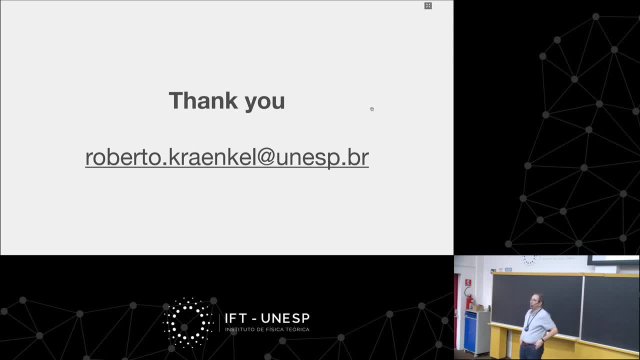 amount of data from COVID Simple numbers. So power laws? no, I don't know any. I didn't think about power laws or Something simple that you would say: there is a power law with a factor 1.2, and then 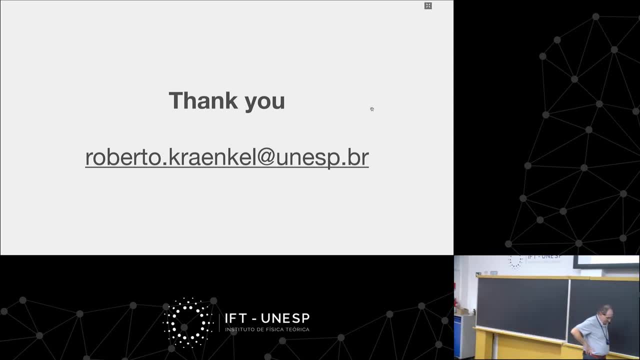 you would try to come up with an explanation for that, Something that is quantitative and that you could say: we have to explain this. Otherwise, it looks like if you have many parameters, how could we compete with Google, Facebook? I mean, these people have hundreds of people working for them. 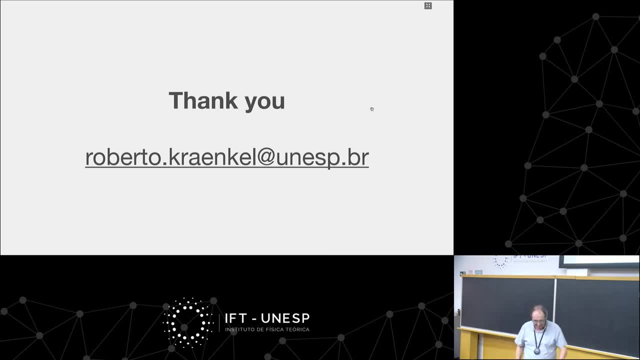 They're super specialists in models. They know all these networks that you are talking about. They don't know all these networks actually. No, No, So, yeah. So what are the people that work with so much data? what are they missing compared? 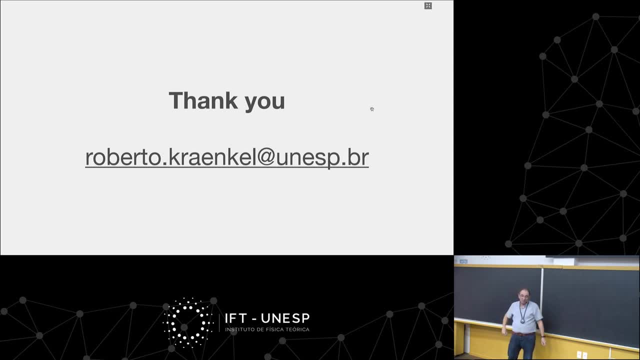 to physicists. So one thing is, people that do have sometimes too much data. actually, For instance, there's a lot of people doing machine learning. okay, And this sometimes misses the point in epidemiology, because you still want to have not very high. 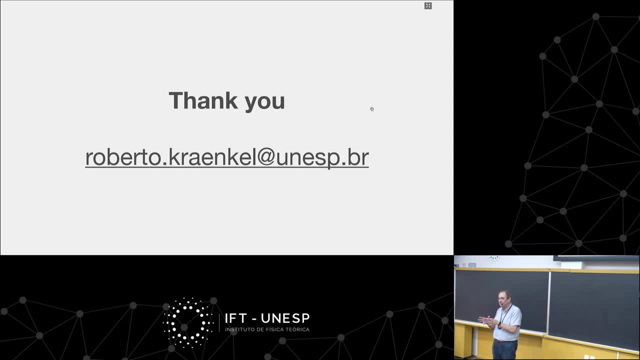 data. You want to have very simple models, but intermediate complexity, which means that you can still- because with, for instance, with too much data, with using this kind of artificial intelligence and things and so on- doesn't give you any insight about mechanisms. 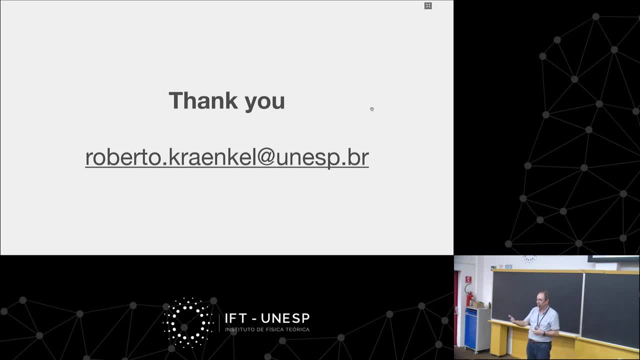 Okay, So you want to have mechanisms to understand what's going on, but you don't want to have it so simple that you cannot explain anything, So you have to have some intermediate range of complexity so that you can still talk about mechanisms. 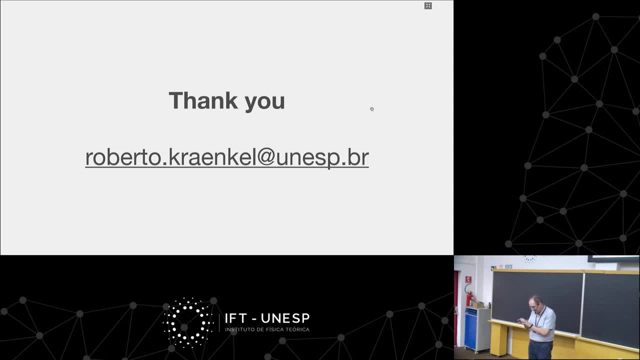 And be more or less realistic about the data, about the model can explain the data, and so on and so on. Okay, I have a question here. There is, I mean, one lesson that I got from your talk was that you can make the models. 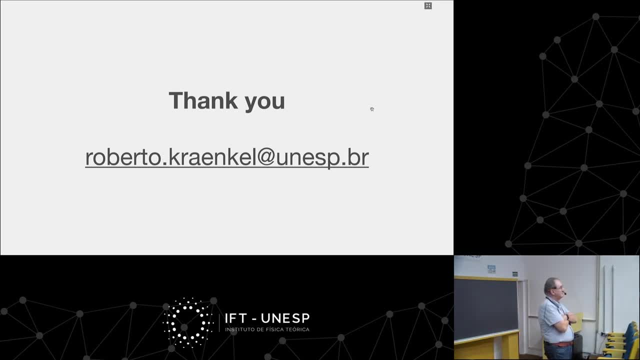 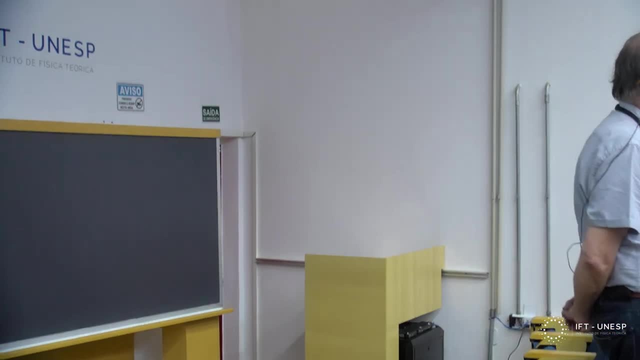 as complicated as you wish, at the cost of overfitting Right. Right, It's the same thing as tweaking often, or something like that, but there is an ingredient that I guess would be important, which is the interplay between different diseases occurring. at the same time, For instance, you can get a flu, your immune system goes down and then you get more susceptible for getting COVID or something like that. What's your personal view of this? Is it being taken into account in the modeling in general, for instance? 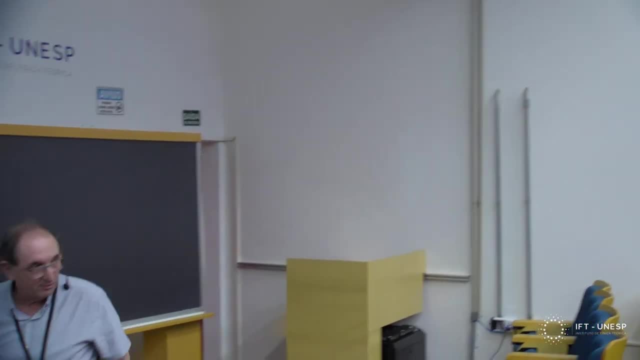 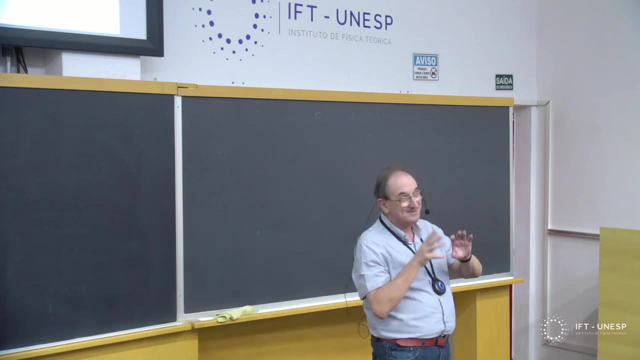 The systems. is this important Or…? MR? So it can be important, yes, Um…. For instance, this is very important in dengue because you have serotypes in dengue. okay, It's not a different disease. but you get immune only for the serotype you've got the disease. So there's a kind of population dynamics of serotypes, of occurrence of serotypes. okay, So you get immune to serotype 1, and then at a certain point there appears a serotype 4,. 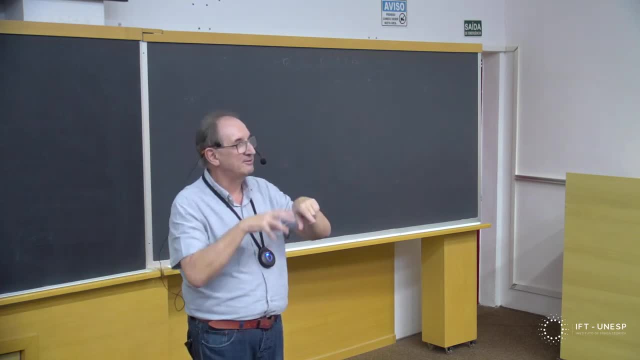 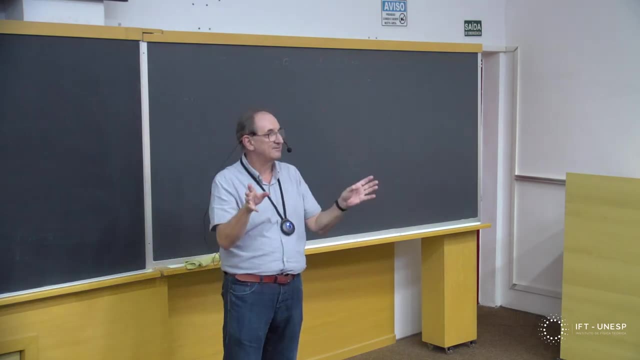 then you are not immune to this one, or you are partially immune, and so on. So there's a competition between serotypes. for dengue, for instance, It's a particular case because there are four serotypes, and so on. 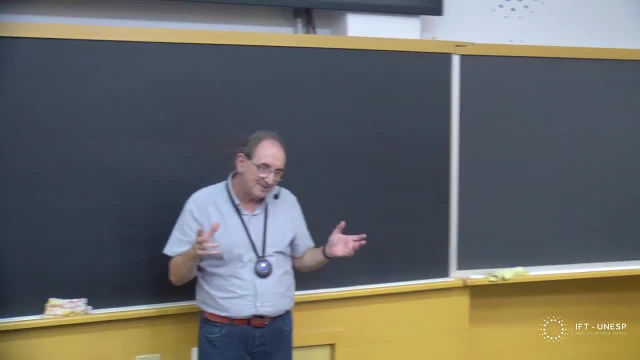 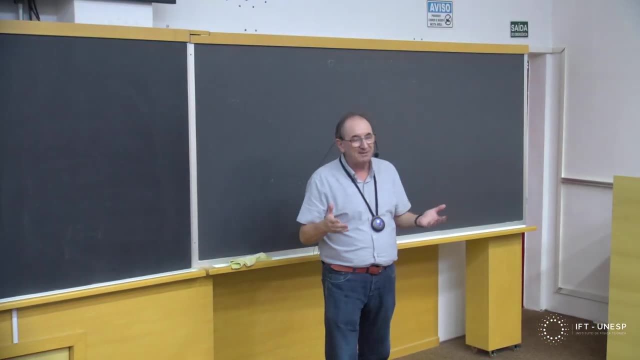 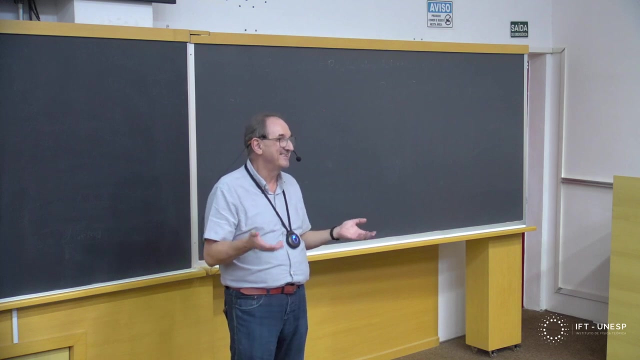 And so interaction between different things- for instance, flu and COVID- didn't seem to have much interaction actually. I mean, there was one interaction that was due to COVID: people stayed at home and then they got less flu also. okay, 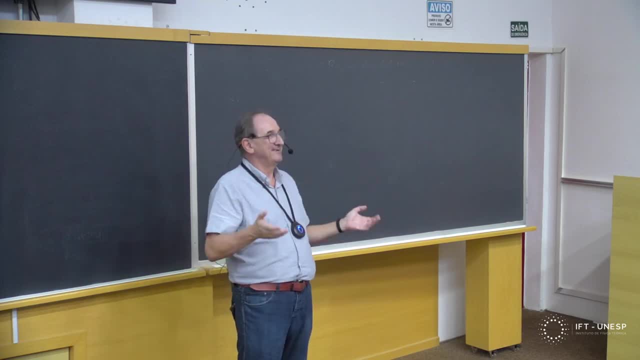 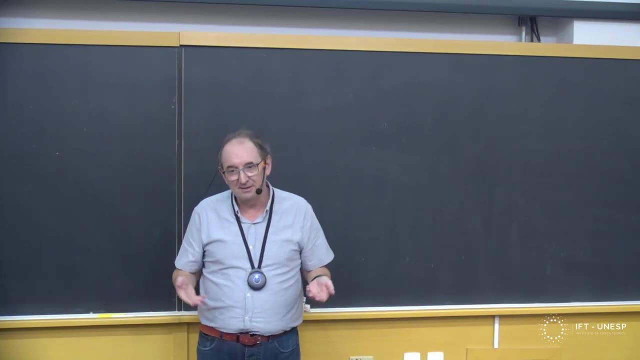 But this is a kind of social media, so it's a very complicated effect okay. But yeah, there are studies about in-host competition between pathogens also, for instance, Co-infection. if you can have co-infections it's different from if you don't have co-infections, for instance. 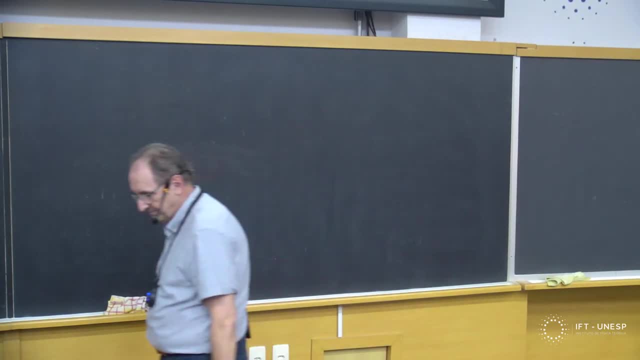 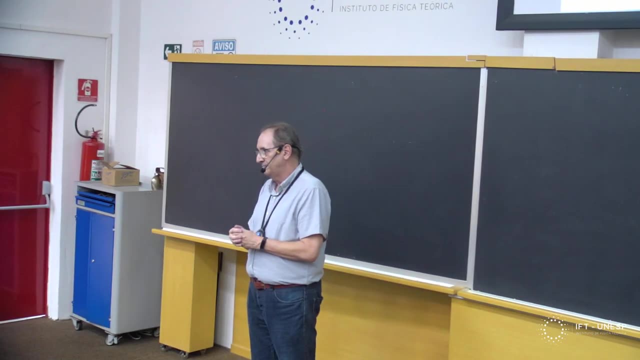 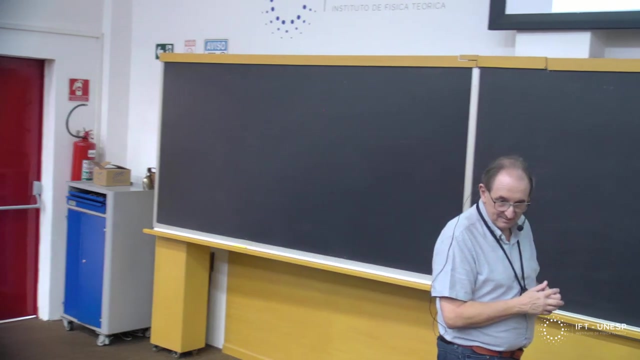 and this changes the dynamics. So can I just ask a question: What is the goal at the end? Is it to be able to predict something, or a posteriori to explain what happened before? Both things. So, for instance, one of the examples I gave you: 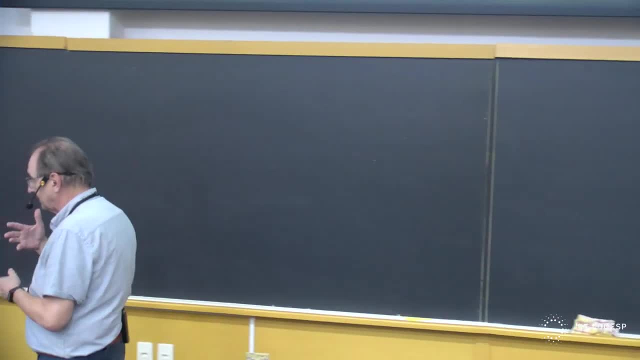 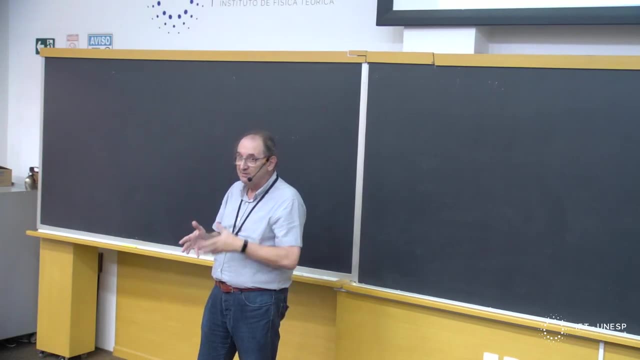 the second one was to try to understand why we could have such a big epidemic in Manaus, knowing the fact that a lot of people already had COVID with the wild strain. So one thing is okay, let's see what's the best explanation. 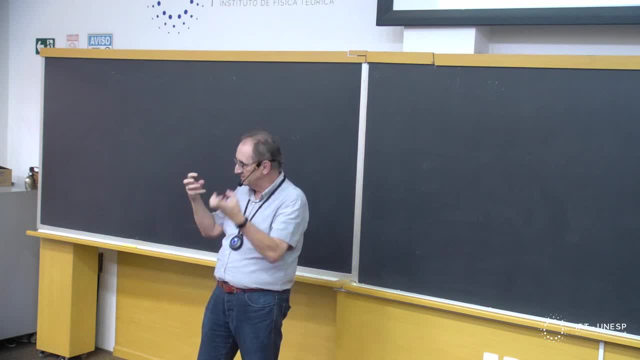 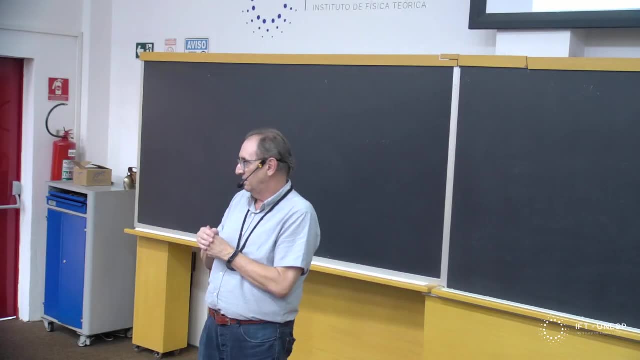 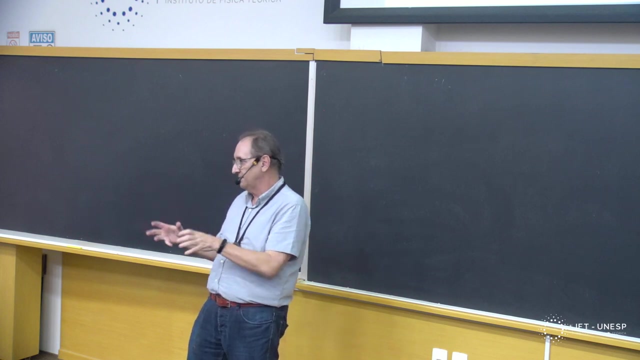 for this number of cases. It turns out that it's a combination of a waning immunity or no immunity against the new variant, together with a high infectivity of the new variant. So that's one thing that's trying to explain what happened. 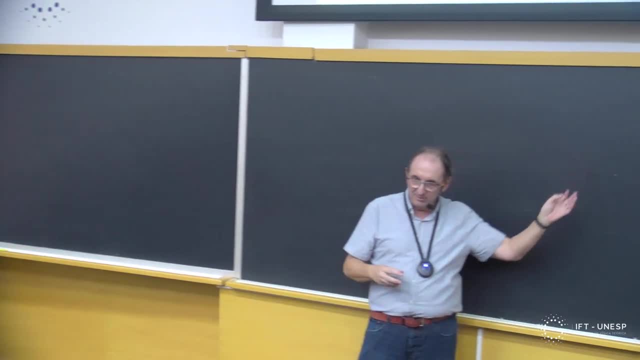 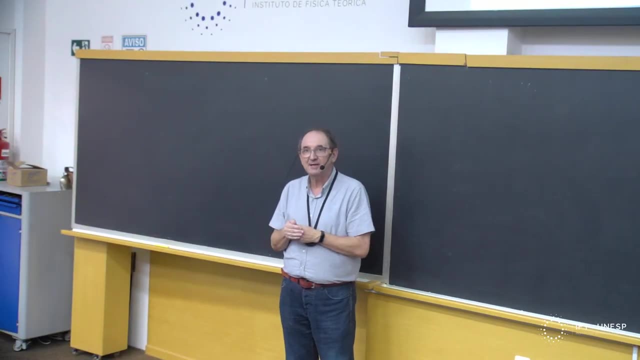 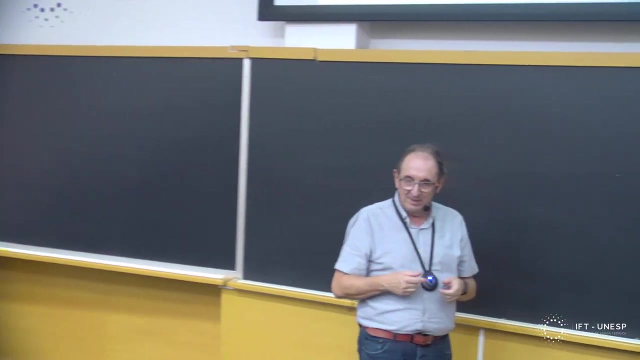 But you can also, for instance, with the now-casting and so on, you can do short-term predictions also. We have also, for instance, we can access a vaccine effectivity and one work that I didn't show you. it is a statistical model. 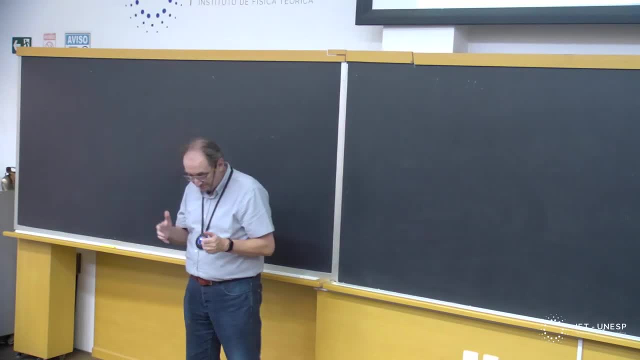 so saying how many in Brazil, knowing the number of vaccines of each type and which effectivity has been used- for instance, in the first months from, say, from January to August 2021, and how many lives have been saved by the use of the vaccines, 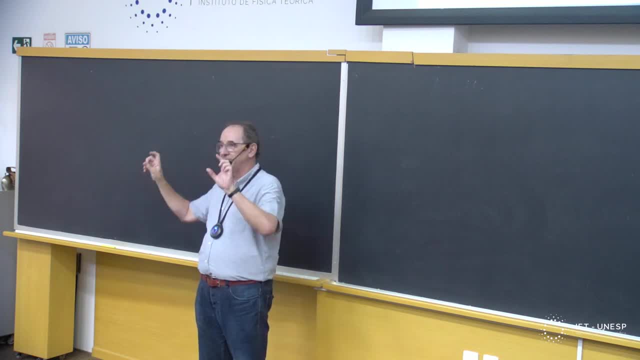 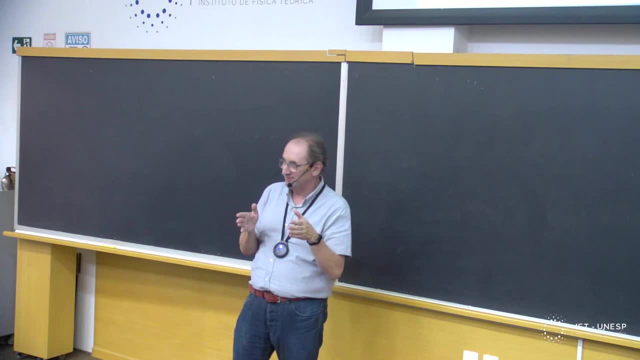 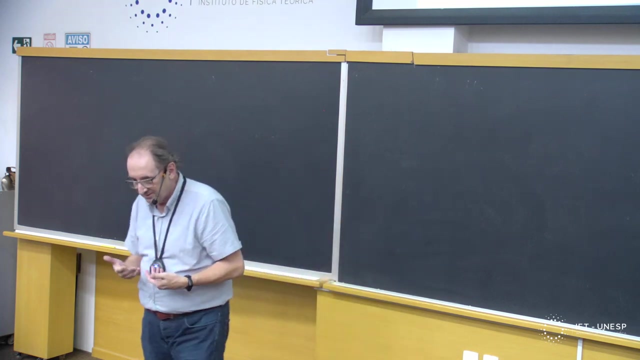 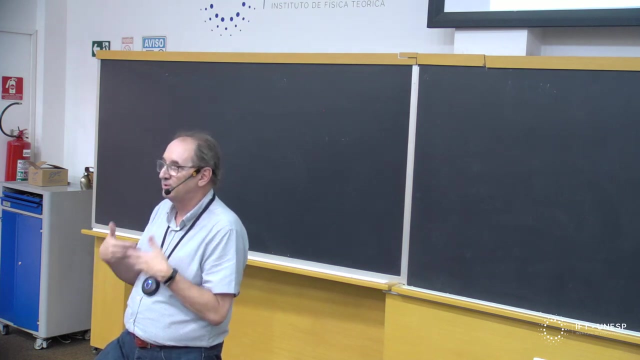 You can calculate this, because they were used only in a part of the population, And then you can also say how many lives more you could have saved if you started earlier. So this is something which is also important: to know how the vaccination in a population has been important. 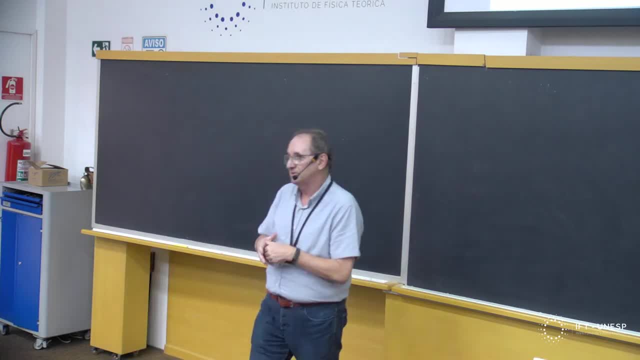 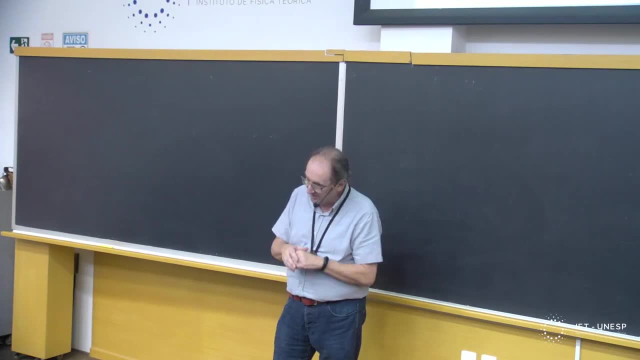 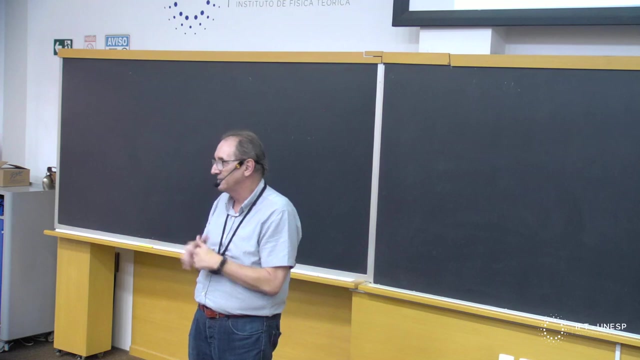 but not how many lives and how many. So this is one thing. that's an assessment of the situation, So long-term predictions are usually ruled out. If you look at the epidemic curve, you'll never predict that, because there are so many effects that you cannot. So long-term? it's not usually. Maybe they cannot because of privacy, but don't you think that, say to estimate where the next dengue epidemic will be, that Google will be much, much better than you could ever be? 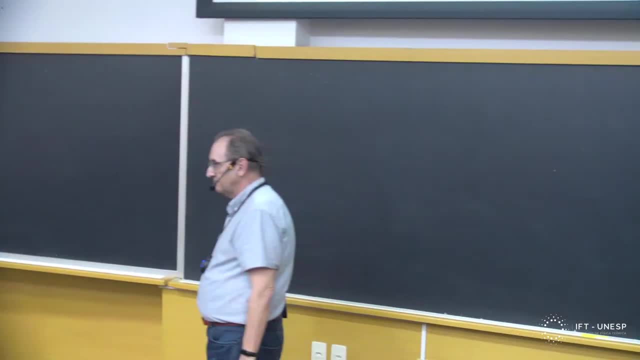 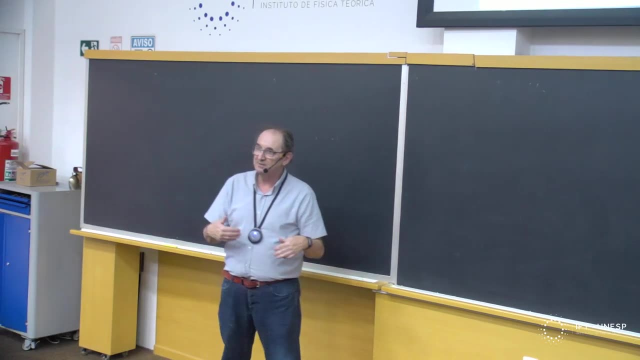 I mean, if they really wanted to estimate, they just need to see when people start searching for dengue. Yeah, you can integrate this. I mean, people do integrate this, actually, And there are people that do the integration of data from Google. 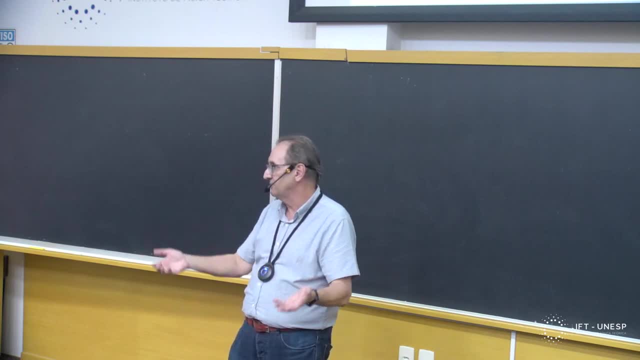 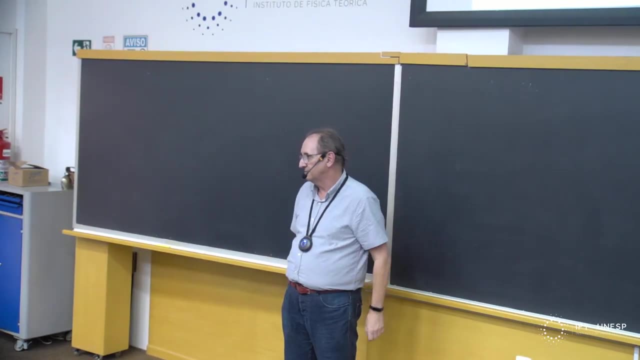 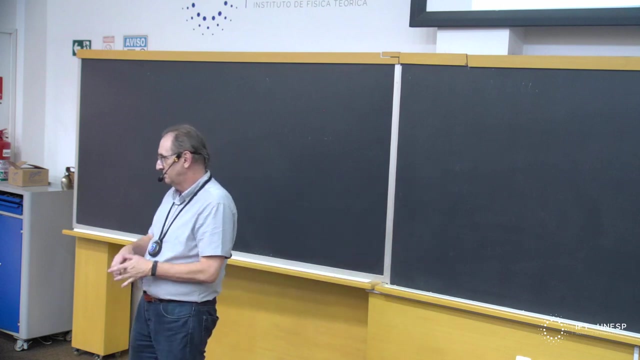 with the data from the field, from actual notifications. So there are people that do this kind of thing. Our group doesn't work with that- but there are people that do integration. That's why I was asking if there's something super quantitative. 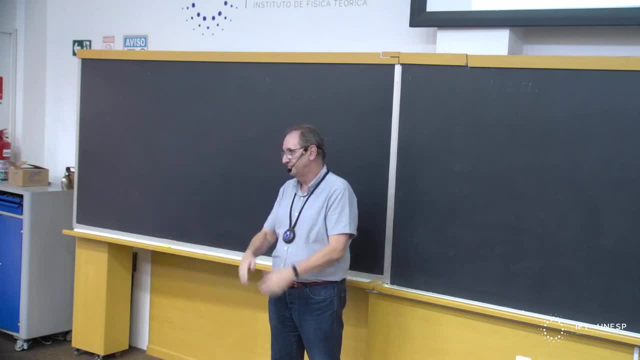 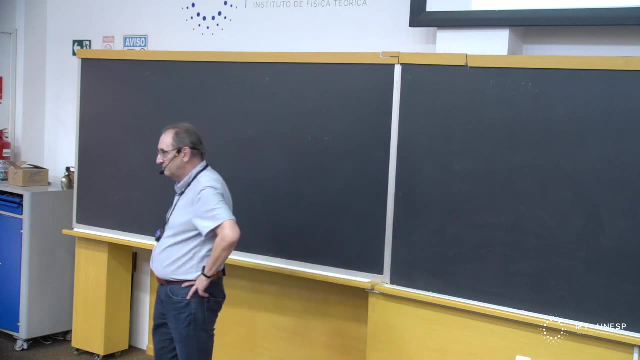 because if it's super quantitative, like a power law or something, then I understand, because otherwise, like the example of Manaus, why could the doctor or a layperson say it's probably because this variant people were not immune. Because then, getting a model that goes past those points, as you explained, 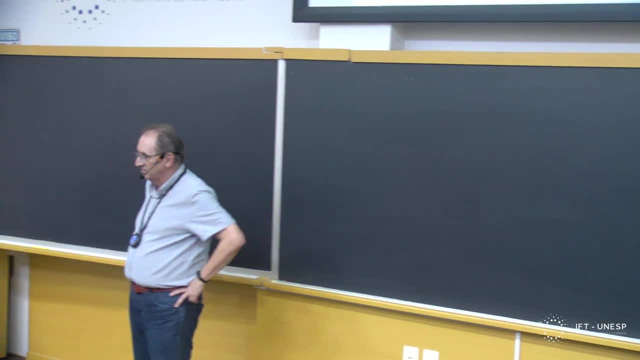 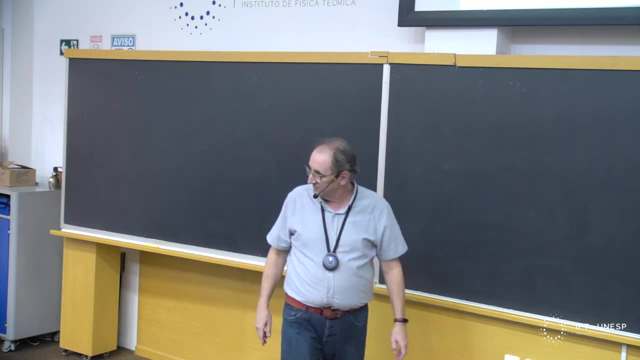 if you put three or four parameters, of course you can feed the Gaussian right. So if it's more or less clear, qualitative, what is the advantage of having a model right If you just say probably this is the mechanism? 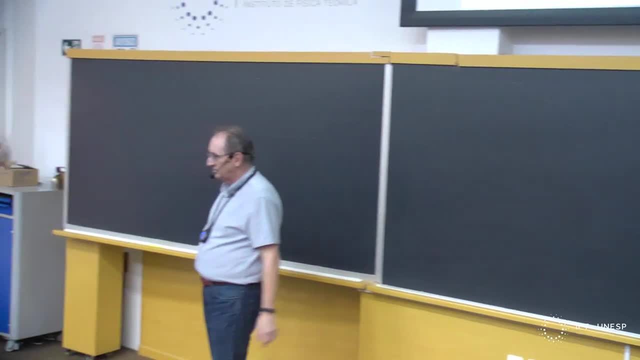 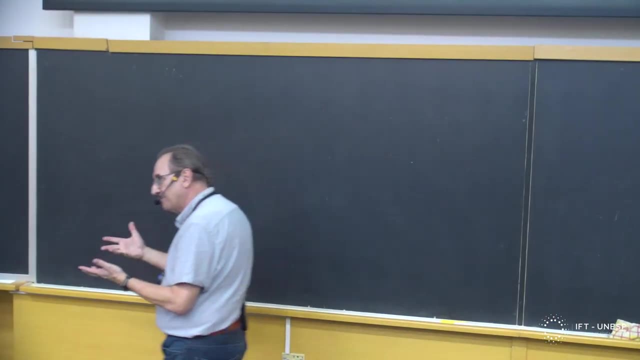 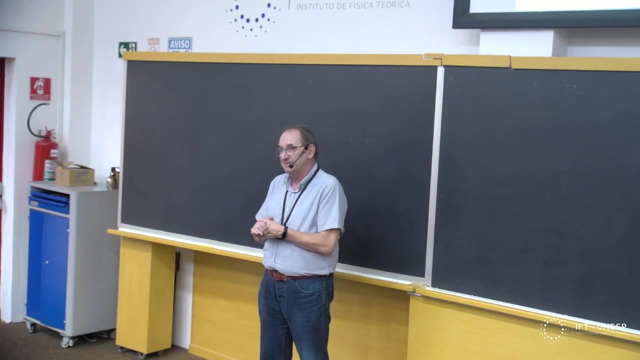 Why is this better than writing some differential equation if they have four or five parameters? So actually we wrote the system of differential equations that have some small number of parameters, to be I mean three or four- And this you showed that it's compatible with the explanations. 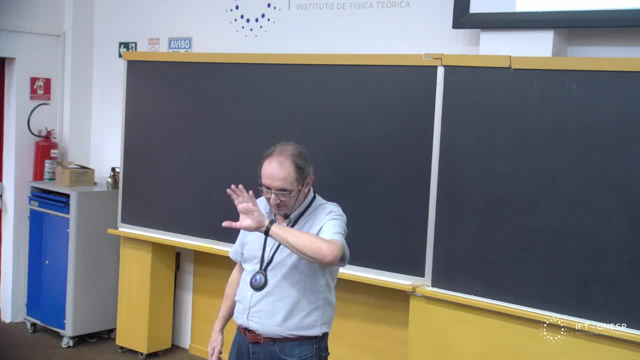 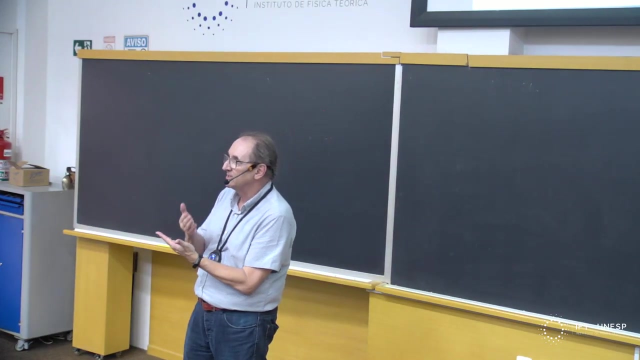 that there could have been immunity. We had immunity before, but actually this immunity was not effective against the new variants. okay, So that's an explanation about. it shows the compatibility of the hypothesis with the data and can be an important explanation. 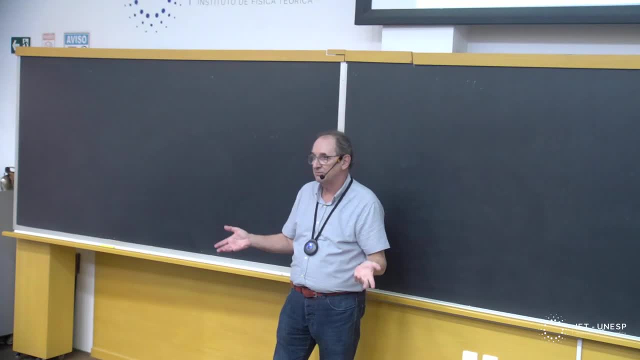 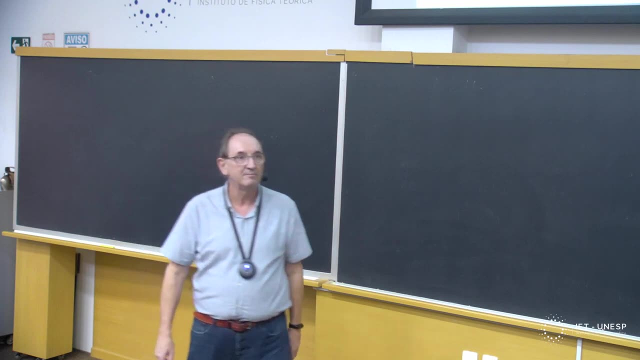 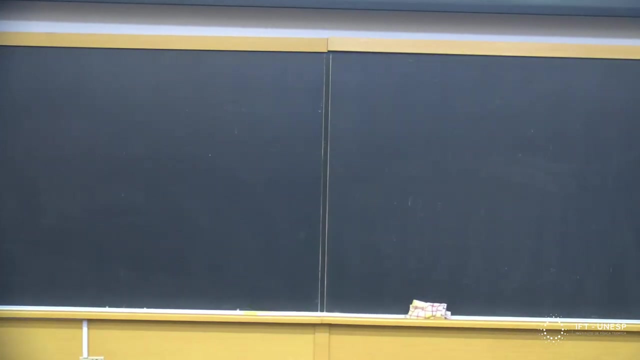 And then you go. for instance, people went to test right And actually it was okay. Good, We have a last question before the coffee break, And concerning prediction about the future, it seems that it's difficult to predict the present. 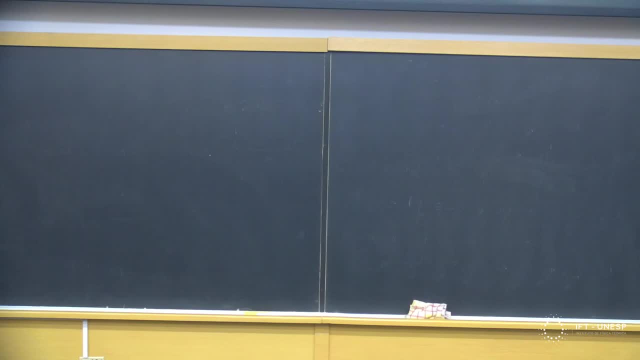 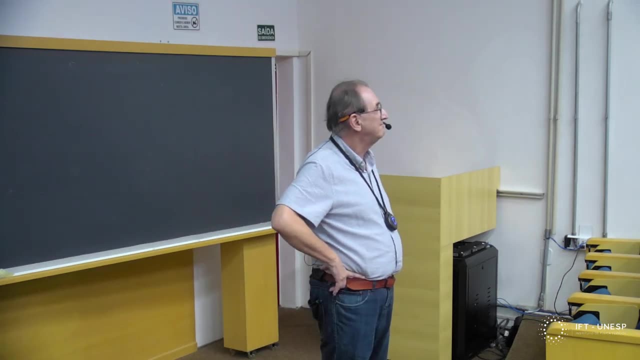 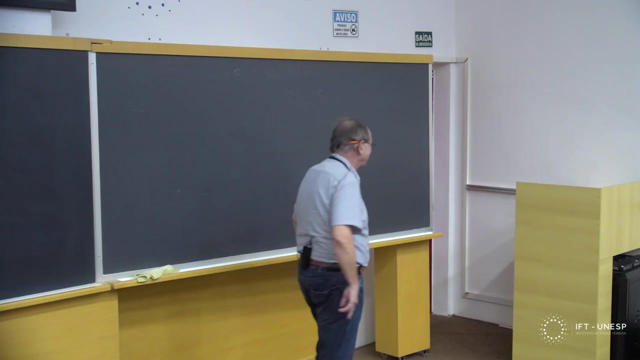 But still, when we see the peaks of the outbreaks, we see that they are smaller and smaller as time passes. Can't you forecast something about the future that the next outbreak is going to be? you know, Yeah, people have tried to see. I mean, our group actually tried to see. 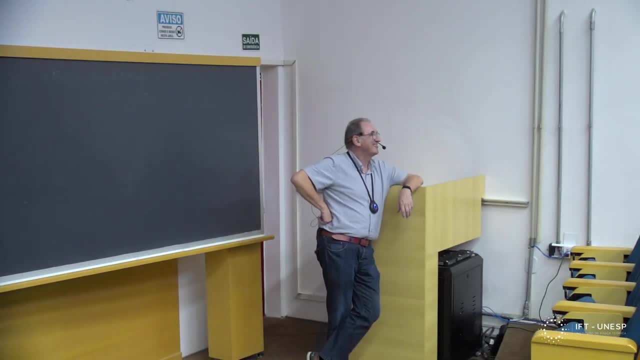 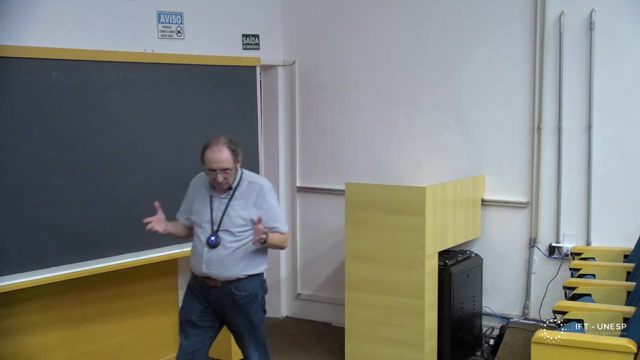 You do wavelet analysis And so it's kind of a sort of thing to see There are some regularities between the. But well, it didn't work. actually It doesn't work. Well, maybe you can make it work.